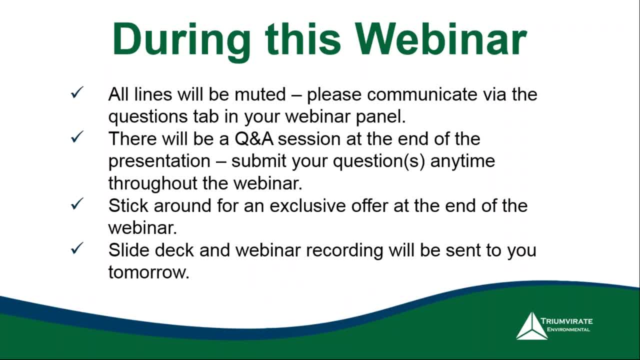 or a technical issue comes up, please use the questions box over on the right-hand side of your screen and I will address your question. Following today's presentation, there will be an open question-and-answer period. A lot of information in today's webinar and I know. 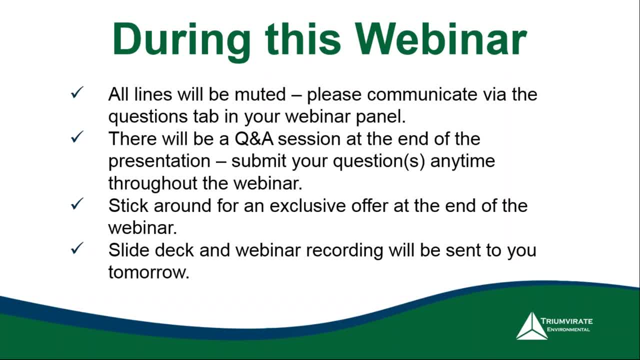 our speaker is going to do his best to save a few minutes at the end for questions. In the event we don't get to them all. we'd love to follow up with you in the next few days, but we'll take as many as we can. Also, we'll be announcing an offer at the end of the webinar. 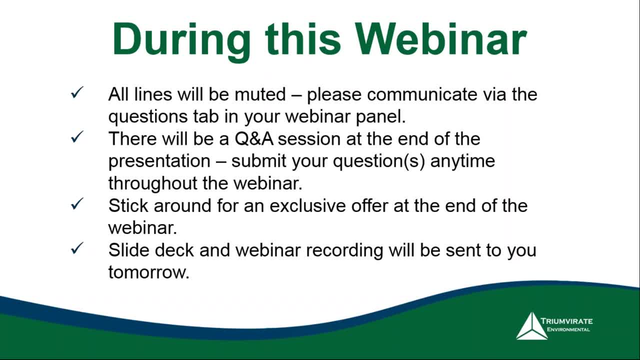 so be sure to stick around for that And, most importantly, we'll be sending you the slide deck and the webinar recording tomorrow. Keep an eye out for that email. Please introduce our speaker today, Rick Foote. Rick has over 25 years of EHS experience and 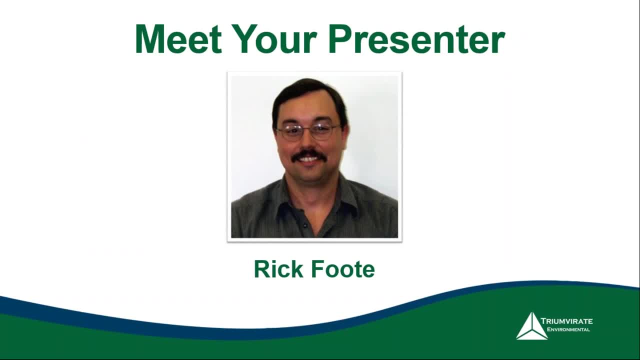 is currently Director of Industrial Practice here at Triumvirate Environmental. Rick has been with Triumvirate for over 14 years where he's established dozens of successful EHS programs for companies that had few or no systems in place. He brings client programs. 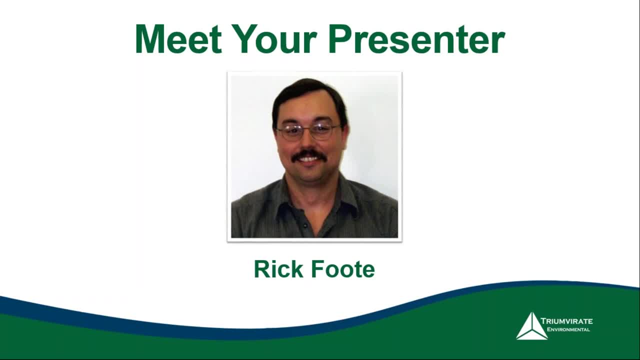 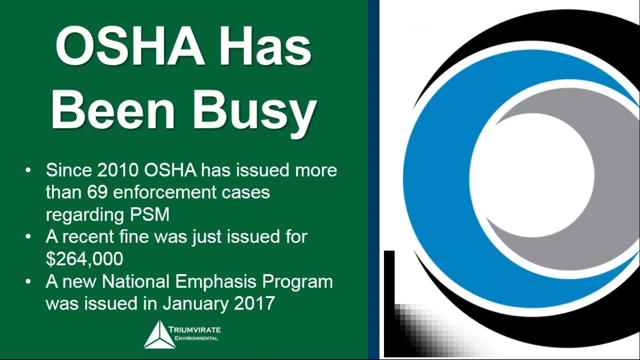 into full regulatory compliance And he's able to customize these programs to individual client needs. And so with that I'll turn it over to Rick to talk a little bit more about what he's going to present. Okay, Thank you, James. Good afternoon everybody. So today we're going to talk about the OSHER. 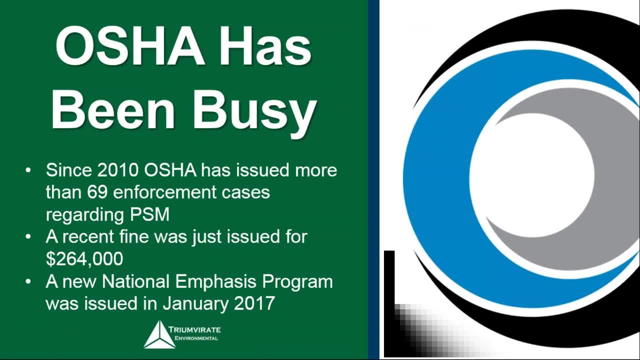 Process Safety Management Regulation And the reason why we decided to talk about this one is OSHER has been busy on this one And you know, as you can see from here, you know the penalties for doing this, you know, are quite substantial. There was a recent one. 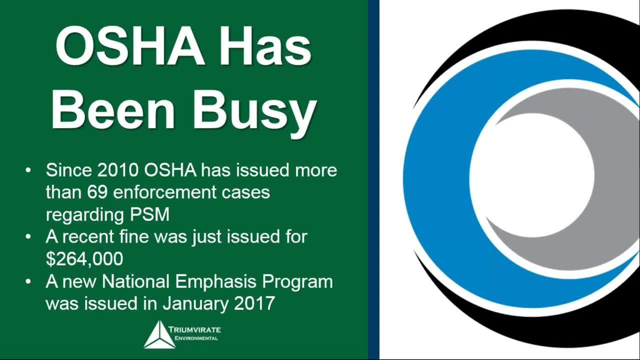 that was $264,000, as well as OSHER has issued a new NEP, the National Emphasis Program, back in January. also around PSM, And as I have talked to a lot of clients, I've realized that some of them, you know, are not aware of the rule or not sure about how the rule 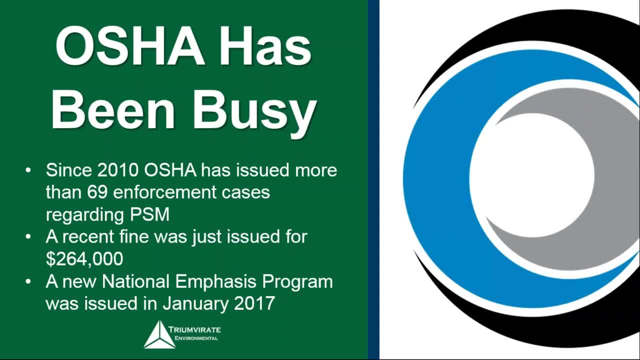 applies to them or if it applies to them. So with that, today I would like to kind of run through. like James said, there's a lot of stuff here, So this isn't a small rule, as if any of you are in the rule know that. So I'm going to try to briefly, as briefly as 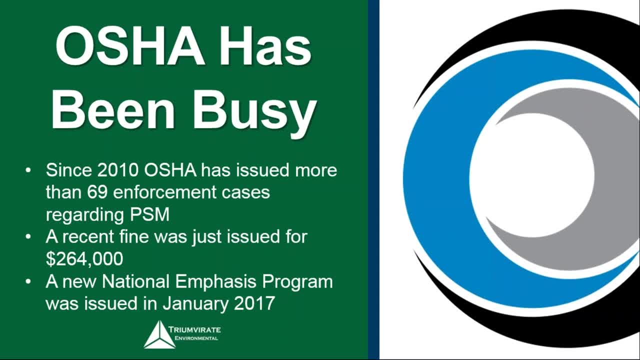 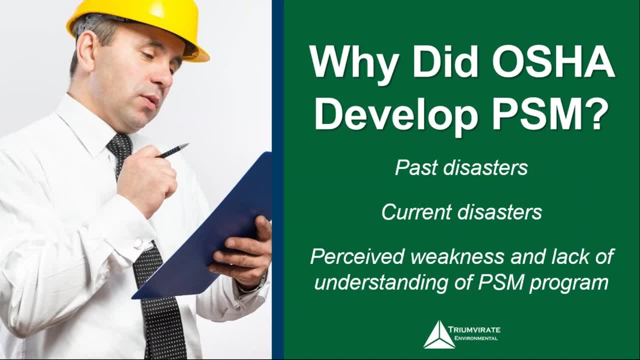 I can kind of just talk about all the different elements of the rule and to see if it's applicable at your particular sites. So I guess we'll start off here. is you know why did OSHER develop this, develop the Process Safety Management Rule? And it really was all from past disasters. 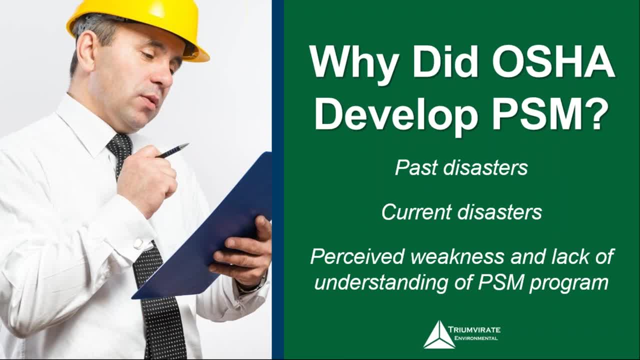 Some of these you know, you all maybe remember, you know, but it really was that and obviously we still have some current disasters And we just had one recently down in Texas with the fertilizer facility, you know, and you know there's been a bunch of other ones also. 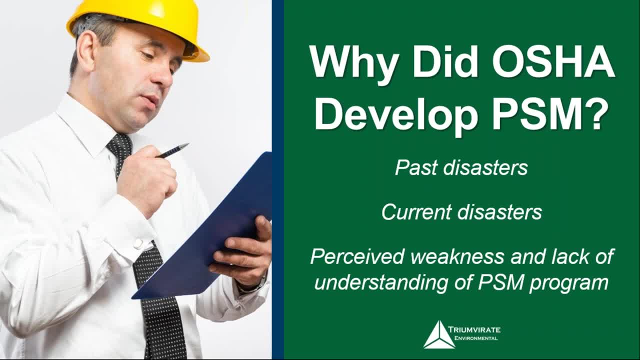 as well. as they revised some of this standard or put the National Emphasis Program in, was because they perceived that there was some weakness within the program. So, in order to kind of flex their muscles, if you will, They decided to say, alright, let's really push this so that people understand it, and 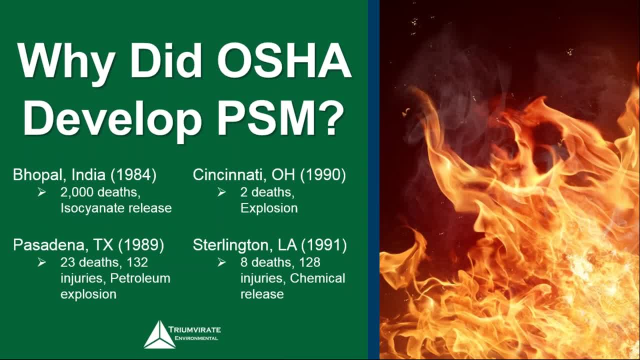 will hopefully do more with it. So some of these disasters, some of them you all may remember, you know Bhopal, India, Any of you that know me. okay, I talk about that situation a lot because I always say that was one of the you know true stories of 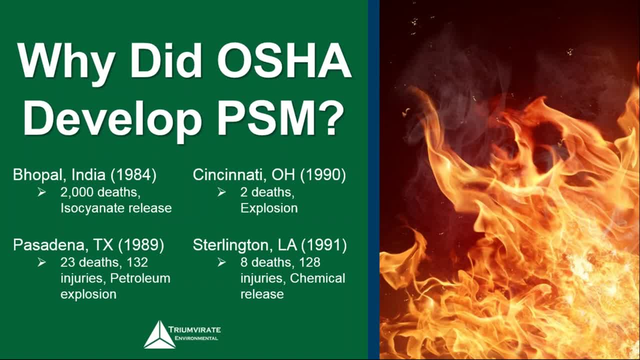 corruption and, unfortunately, deaths, and you know some people call it the first terrorist act of modern times. you know, one really was a big one. you know, all the way back in 1984 was also a great book right by George Orwell, and you know I have a few other ones up here too. and 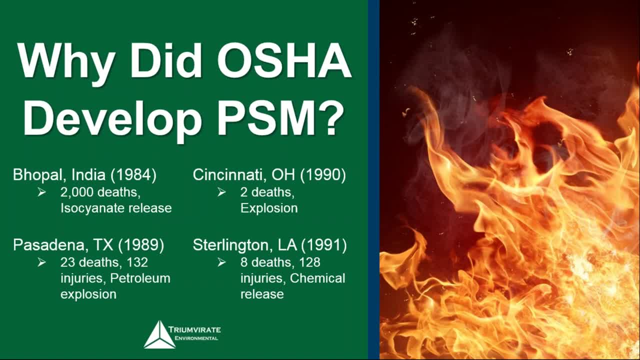 you see that you know really why. you know why does OSHA write any regulation, right? I always say, is you know, here in the United States and we proactive, are we reactive and truly we're more reactive, and this was definitely a reactive type of regulation is to say, hey, we got to do something here to 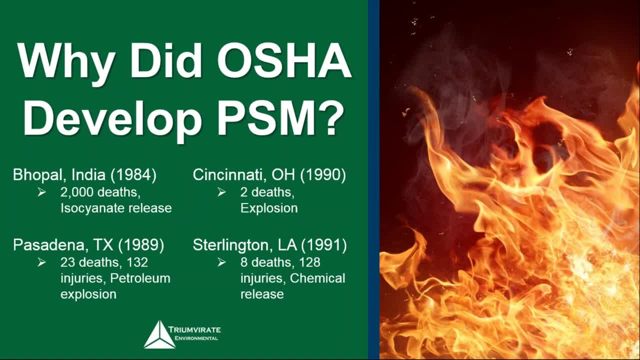 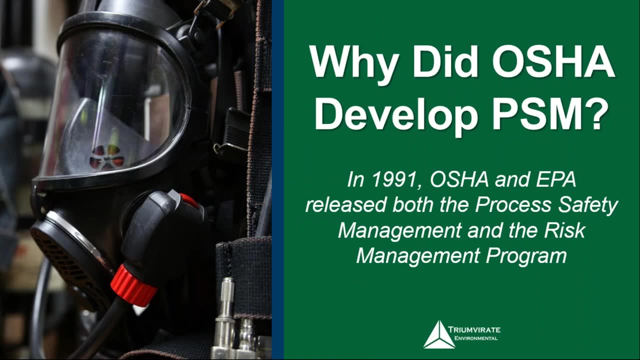 ensure that we're protecting not only workers but people that surround these facilities where the types of materials are being used, so it was a combination type of rule. I hear this a lot too, though, because back in 1991, when this rule was released, you know, we also got the risk management program out of the 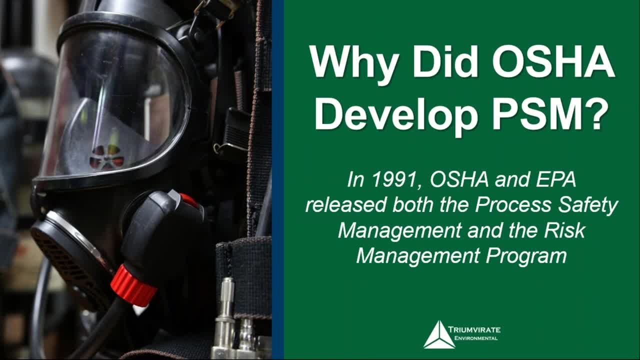 Clean Air Act was released both at the same time. they are distinctly different in many different ways. so I'm really- you know I'm not going to go into too much detail on that right now, but I'm really want to make sure that everybody here understands I am focusing strictly. 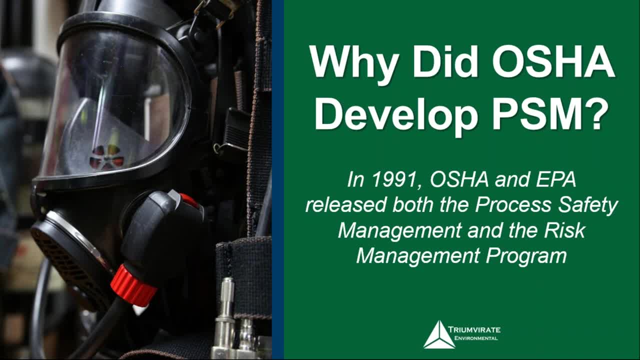 on the process safety management part of these regulations and really not too much going to talk about anything with the RMPs, even though if there is enough of an interest, you know, as James said, we can always do that at a later date- but I really really wanted to take the time and focus more on you know what do you? 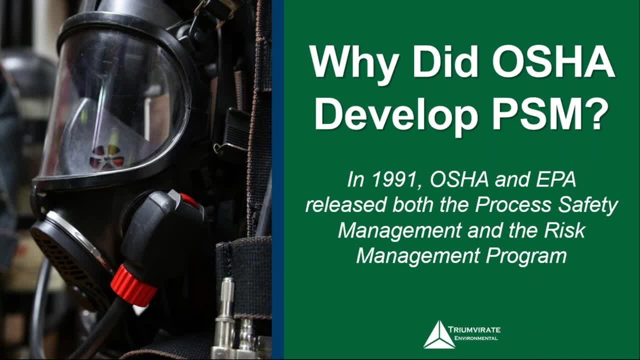 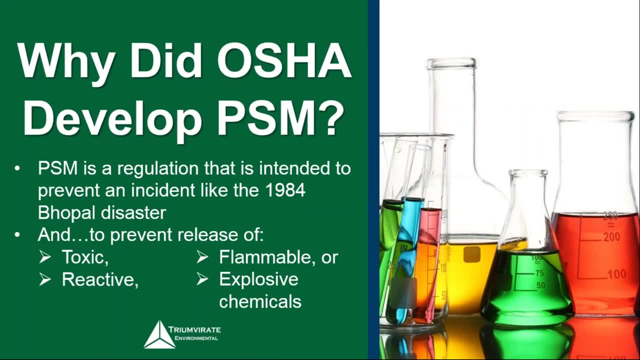 need to do and how do you do the evaluation first, which is the key to understanding this program, is the applicability of it. so when they put this all into into place, the whole idea of the regulation was intended to prevent things like Bhopal or you know. 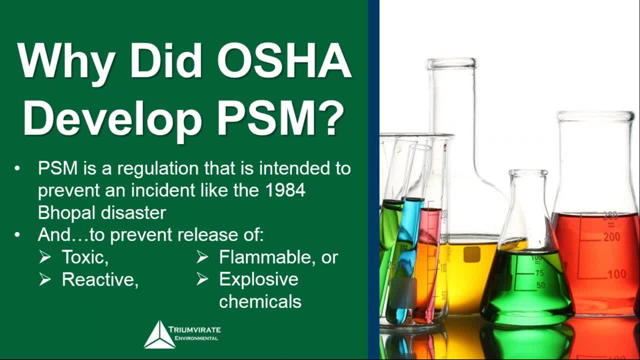 any of the other incidents that you want to talk about, and it was, you know, all around the toxin reactives, flammables and corrosive chemicals, you know. I mean you see that a lot of facilities or even certain states have already enacted kind of- I call it- Bhopal. 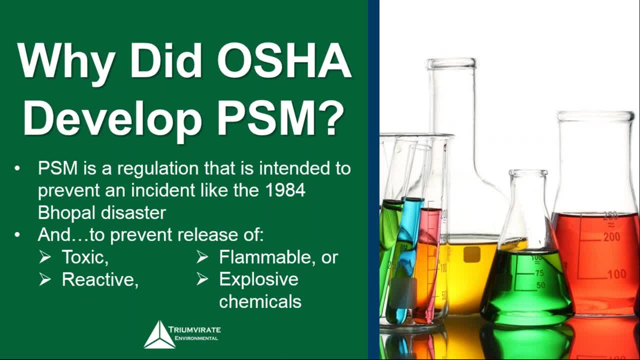 I call it quasi PSM regulations, where they've added to it like where we're from or where I'm from- Massachusetts. you know they have one here too- that they call it a process management regulation, which is different than OSHER's, but it's very, very similar in nature. but it's all about how the materials are used, so it 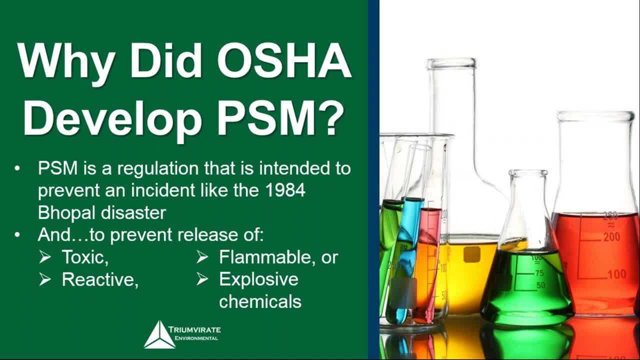 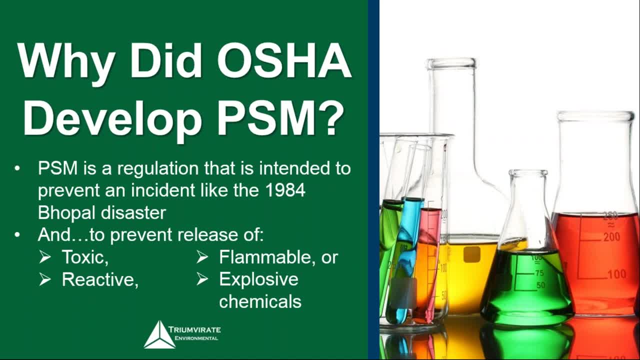 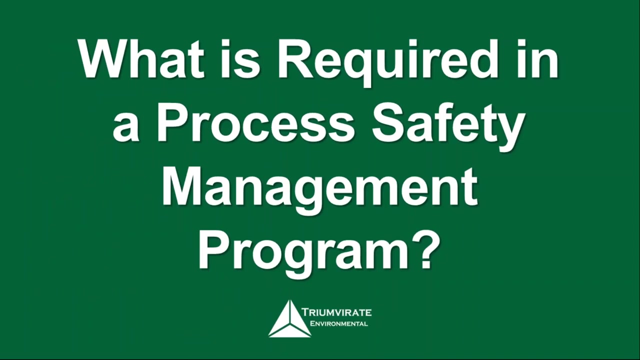 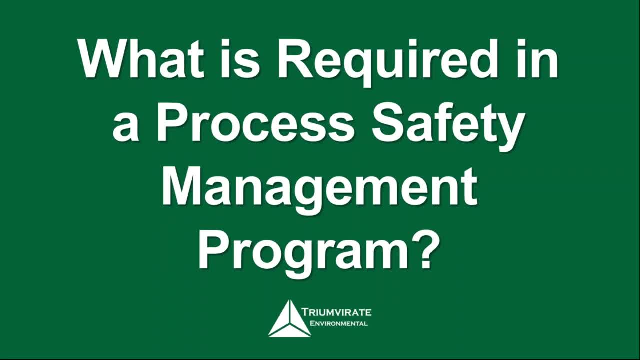 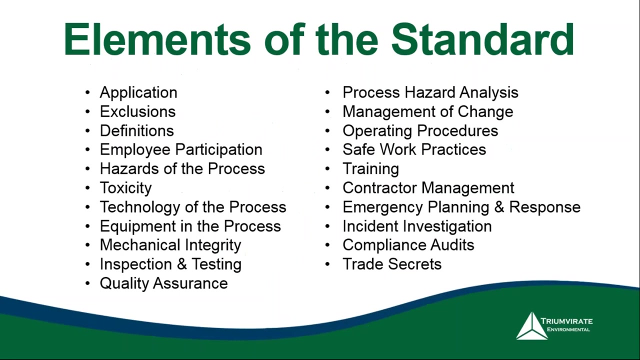 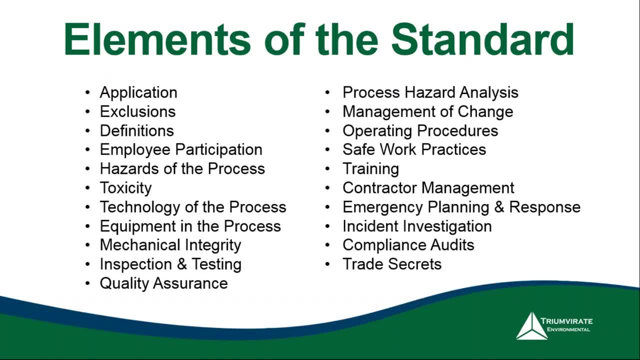 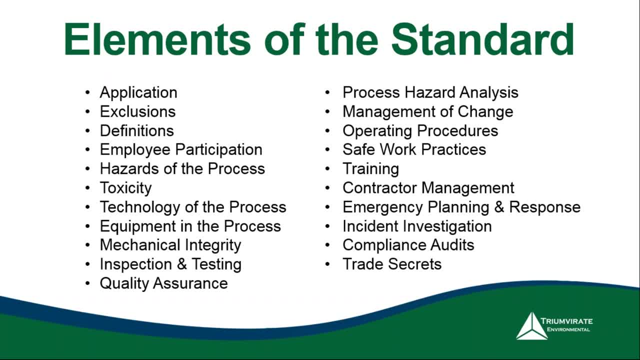 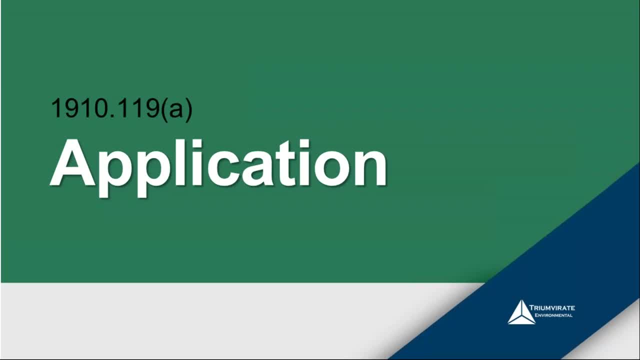 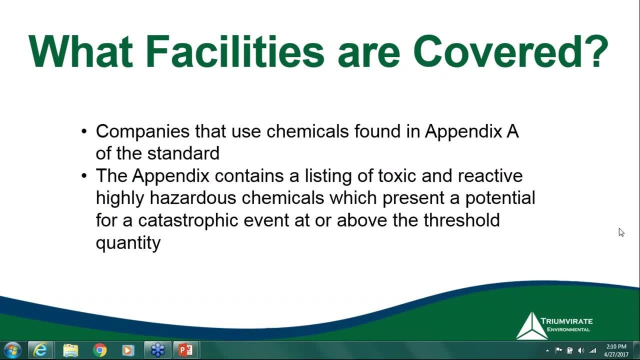 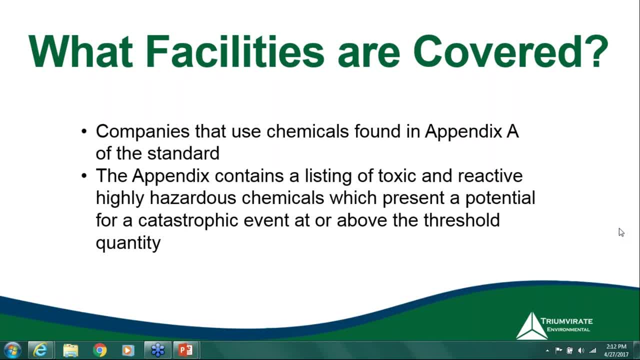 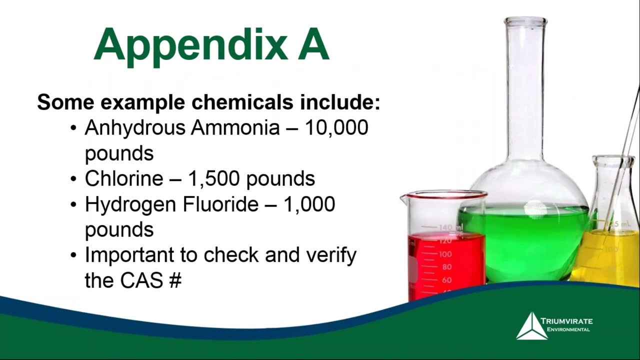 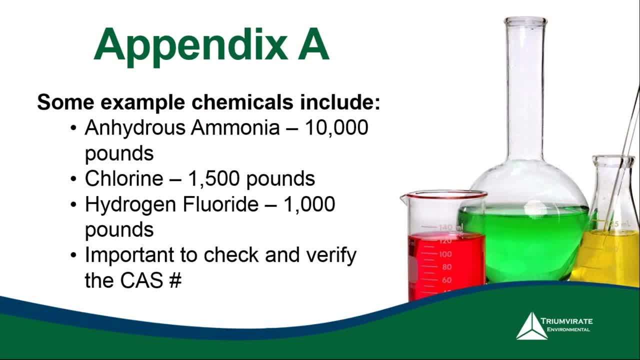 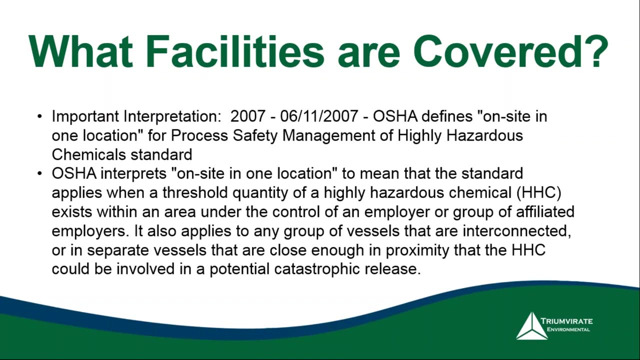 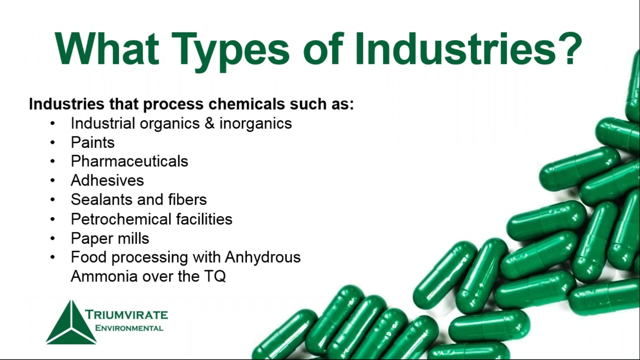 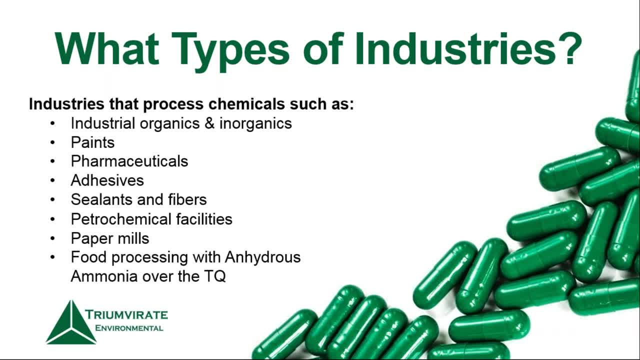 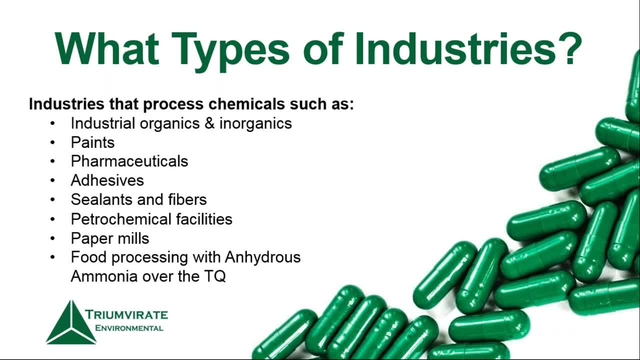 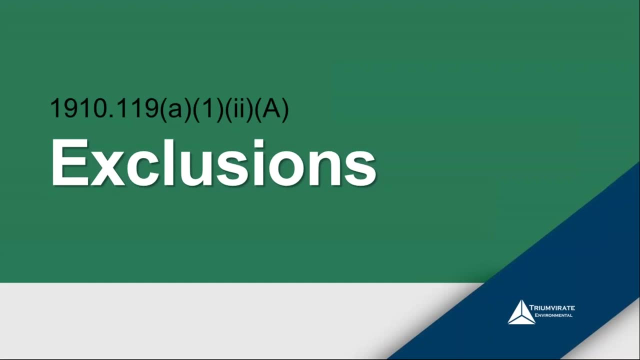 own and what are you responsible for? because it could drag you in, you know, without you even thinking about it. I just want you to look at the entire facility and not just one piece of it. so, with any rule, right, I always say: everybody, who? how do I get out of this? right, because I don't want to, I don't. 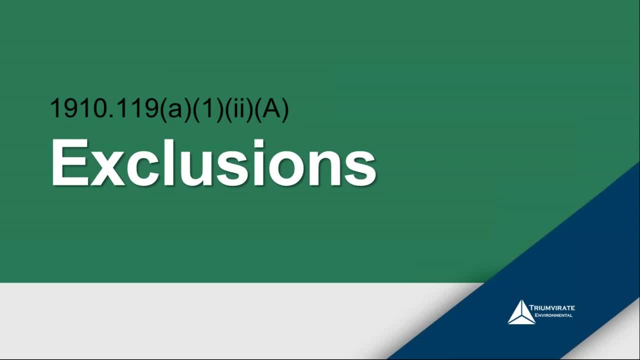 want to have to do this and trust me, I you know, I always say to people: this is one of the rules you don't want to get into because of the complexity of it and how many different things that are really really involved. so in the rule it 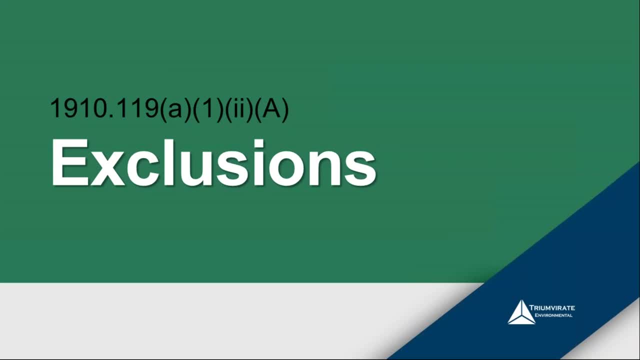 actually gives us some exclusions, and I'm not. you know, we don't have the time to go through all the detail of all of this, so I do want a precursor, as we go along here to say: you know what? I just took out small pertinent pieces that I 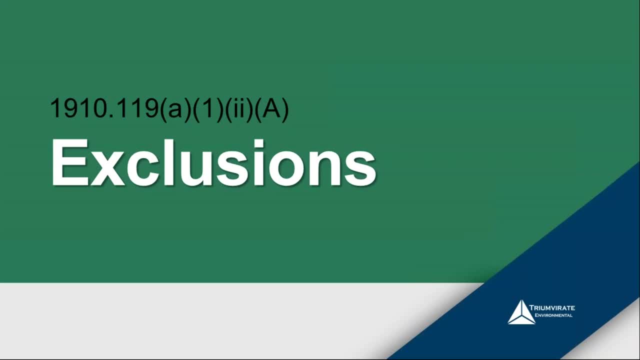 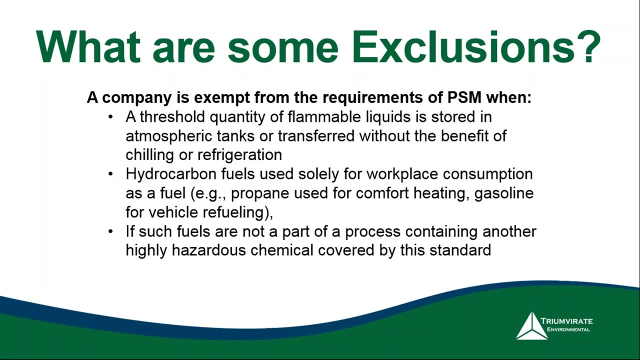 thought were very important to at least begin the discussion here on this so that we're all okay with that. and so with that is you know there is some exception. you know you are exempt from the requirements when you know again it's calling out specific materials, right, flammable liquids. you know again if 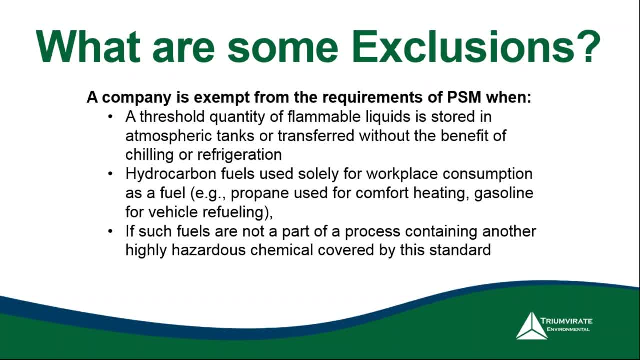 they're stored in an atmospheric tank or transfer without the benefit of chilling or refrigeration. so it kind of says, okay, well, maybe you can get out if. if you have that flammable liquid and you know that, I would say you know, there's a little. there's always more information that got to go along with. 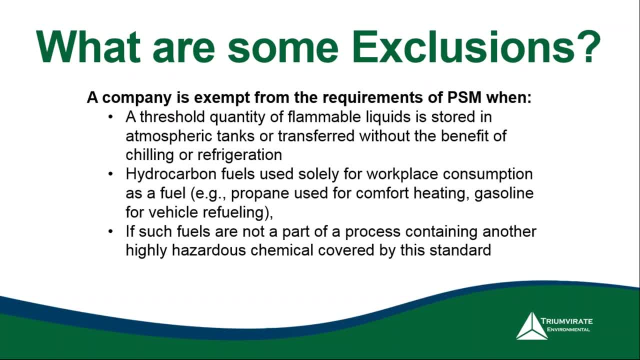 some of these. but it is a great starting point for you to start with- and I think that's a great starting point for you to start with to say, hey, this may work. you know, I might be able to get out of it again. you know, kind of a very similar to a lot of other rules, right, if it's there for as a 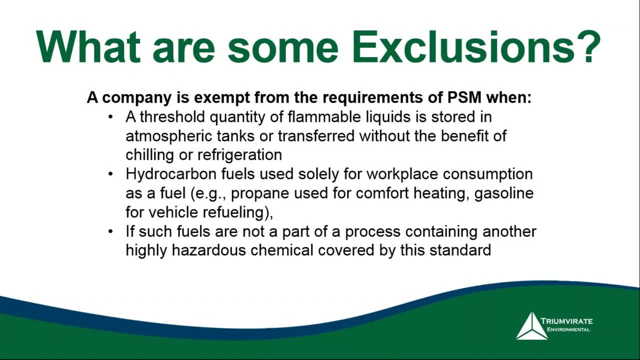 fuel, you might be able to get out of it okay, but if that fuel is going to part of a process you know that's covered by the standard, then you may not be included in it. so I am saying that you got to really look at every single part of this before. 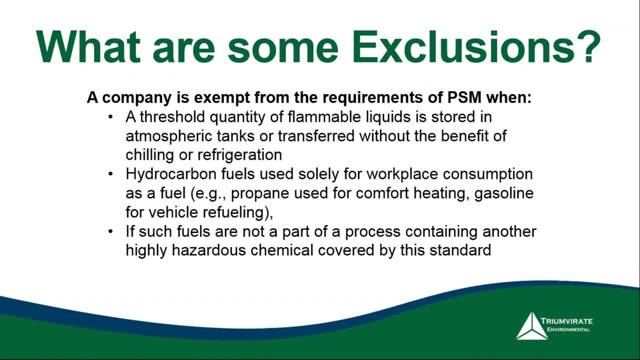 you can say: okay, you know I'm out or I'm in. is you really really want to rip apart that chemical inventory? how is it used? I tend to like to say to start is really okay. figure out what chemicals are applicable to you. do a process flow? 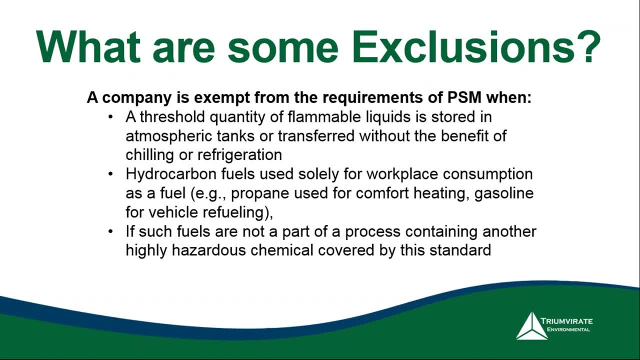 diagram about how that material is used throughout the facility. then come here to the exclusions and say, okay, can I somehow find my way to get out of this? and, you know, do it within the rules and checking other letters of interpretation to say, yes, I am okay. so that is something that's kind of a great starting point for you. 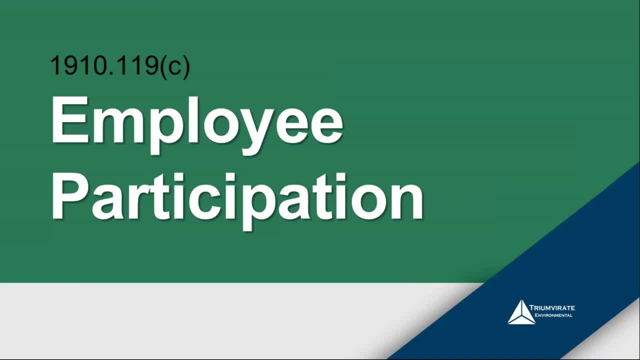 you know you may want to think about. with that said, okay, if you decide or determine, I should say it wouldn't say decide right, that's definitely a bad word. I don't know why anybody would decide to want to get into this program. but let's say you're into it. one of the first things you really want to do is: 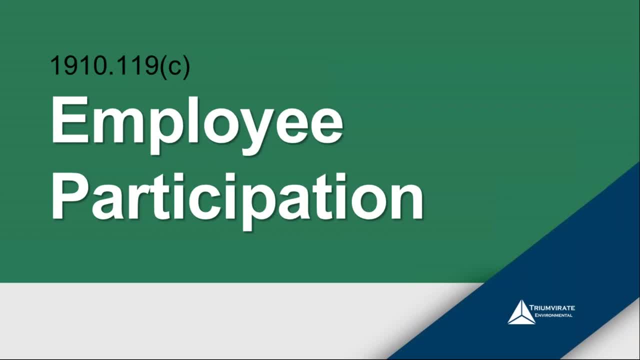 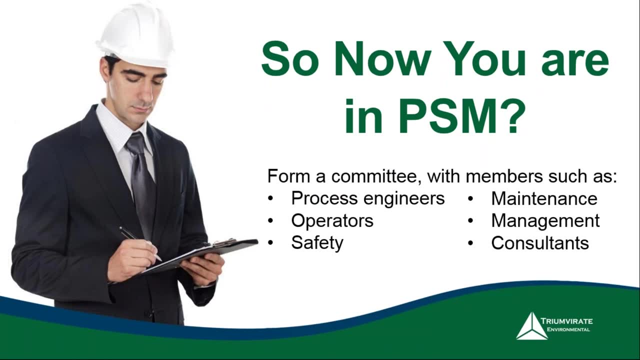 and you're required to do this is to get employee participation. so very similar to other things that we, you know, we always say here: you know you want to form a committee, you've got to get people that understand all the different elements within your facility and that. 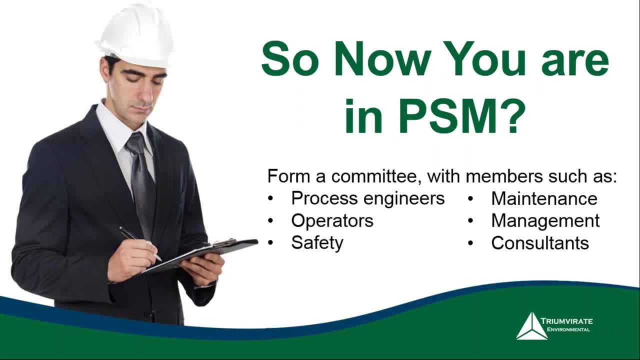 is. you know you want to get people like process engineers. I always say the operators. the operators are the biggest key, I think, within this program is because why they understand it the most. they understand how, what things go on, what could go wrong or what has gone wrong in the past, as Jay said. like I've 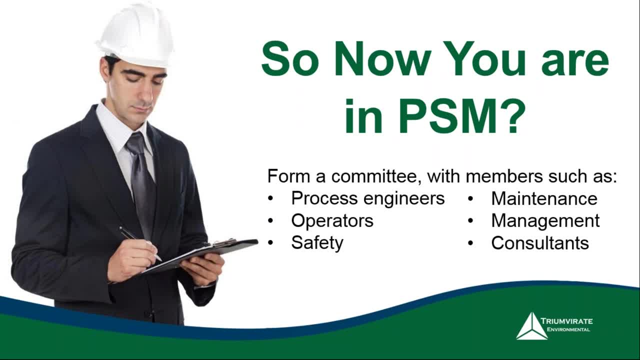 been here trying for a long time. I always say to myself, wow, I got a lot of- you know- historical knowledge about here. so those are the types of people, too, that I want to talk to you at a facility to say, hey, maybe they had a minor incident that involved one of 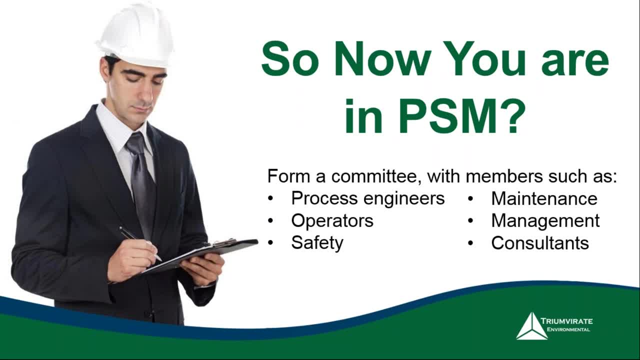 these chemicals, but it could turn into a major one. that's something you want to have. you know the discussions all about and obviously you can see the other ones here. you know maintenance. you want to have management. you want to hire outside help. you know to do this with you also. just some ideas, and I'm sure there's a 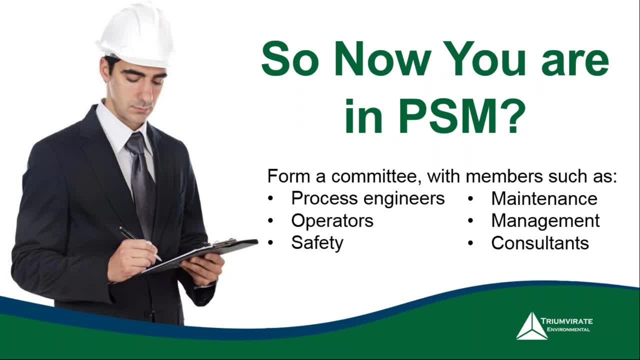 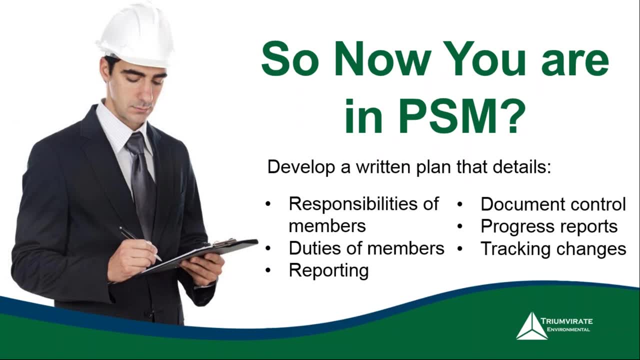 lot more other people that we could add to this slide deck here, but right now it's a good starting point at least. so from there you have to write a written plan, so part of this is is, again, it's process safety management. so you got to have everything in right. how are we going to do it? I always, you know. 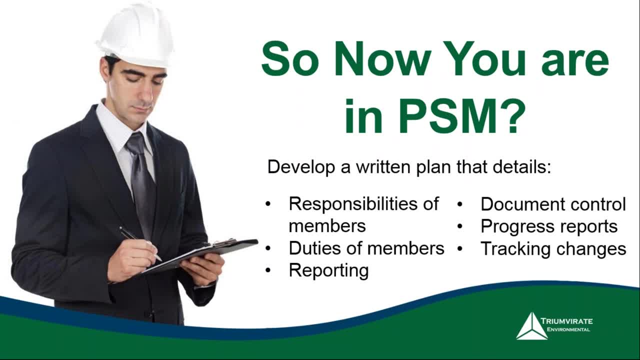 I'm a Three Stooges fan, so I always say: do we cheat them and how right? how do we document it? and also, how do we say that we did it if we don't put something in right? so when you're developing the plan, what you want to do is you want to 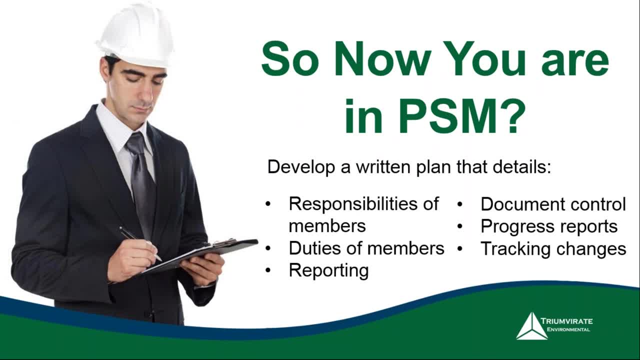 outline what's going on in the plan. right? how does that plan look? right, you want to see it as a process where you can say, okay, we're going to come up with a plan and then the process we're going to do is we're going to write it down and all. 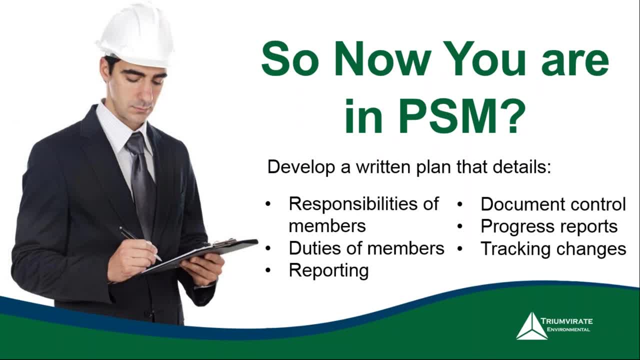 right then, when you're on the line, it's you know we're going to try to get it all right, and so what are we going to do with the plan? you know what are the responsibilities. what do you expect the people of that committee to do for you? 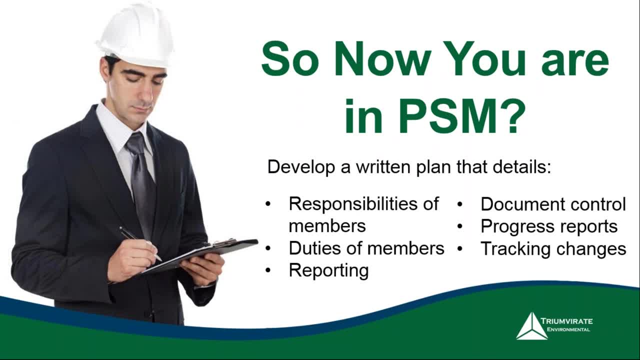 okay, and then what are their duties? what are they going to be? what type of reporting? how are they going to report back to you? how are they going to get you information? and you have that type of document control you've got to set up like progress reports. where are we at? when are we going to be done? where are we? 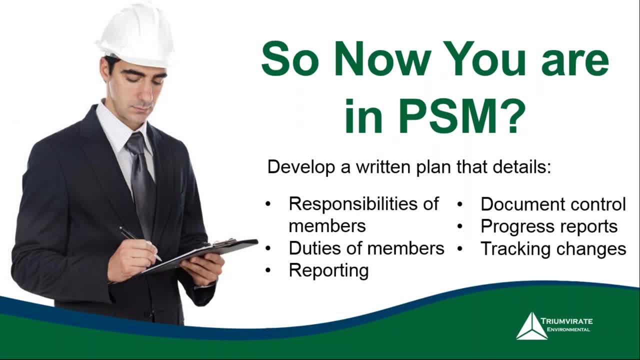 going? how are we going to get there and how are we going to track all of these other changes? you know, maybe it's personnel, maybe it's committee members, maybe it's, you know. again, like I said, change of chemicals or change of process. you want to have a program or a place inside of it to be able to say: yes, we. 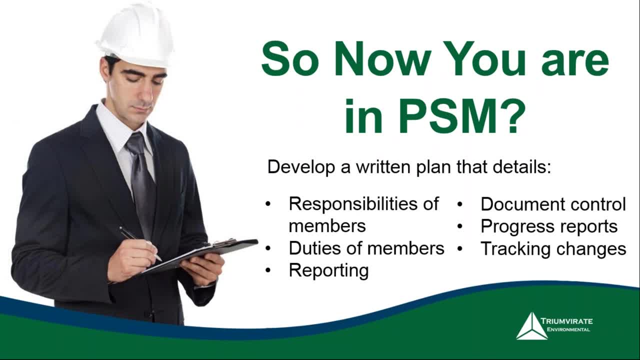 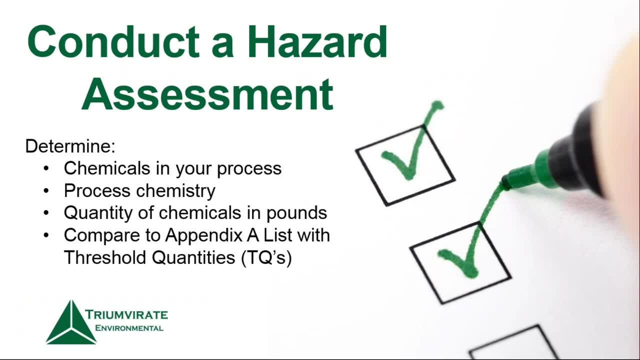 did this, we got it all right and we know what's there. from there, you know you've got to look at again. do this hazard assessment, which is all about alright, what do we got, how do we do it, where is it? and then compare it to the 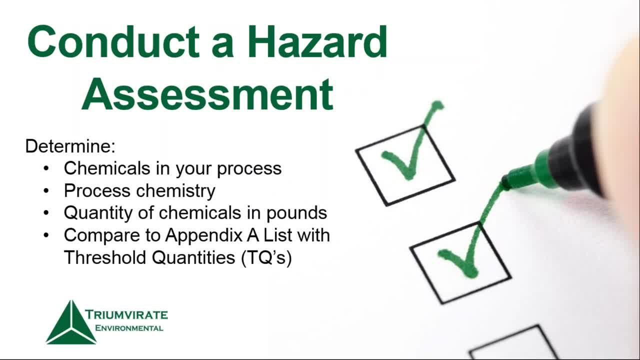 list. it really seems so basic and simple. I think this part of it. but this can be the most complex part, because you know that we get. you got mixtures. you got other things too that wait a minute. we got to trigger it based on this, that or 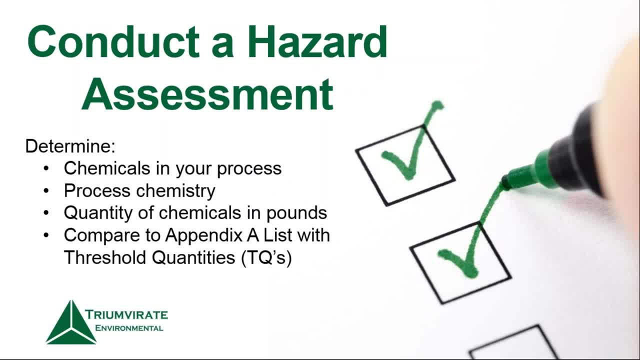 the other thing. so you really, really, really got to get in the nitty-gritty and in the weeds here to make sure that you've collected all of the right information. and then, once you got the volumes of the information, and then you can move forward and say, okay, now what do I got to do with that information? so with that, 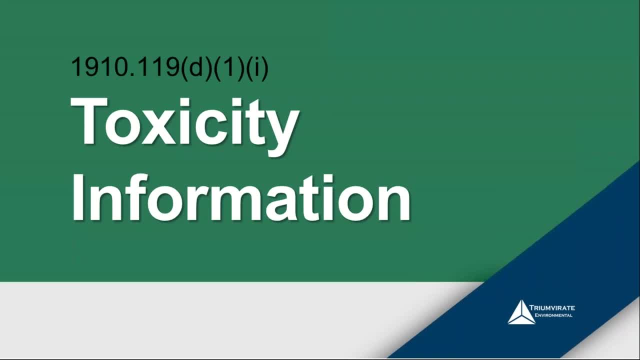 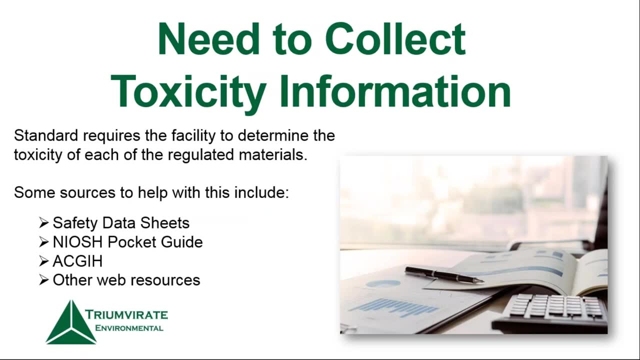 said, it comes into the next part of this, which is collecting the toxicity information. and with the toxicity information, the standard requires you to determine how toxic is that material that you have. and today you know again. you can remember back when the rule was originally promulgated. you know, we. 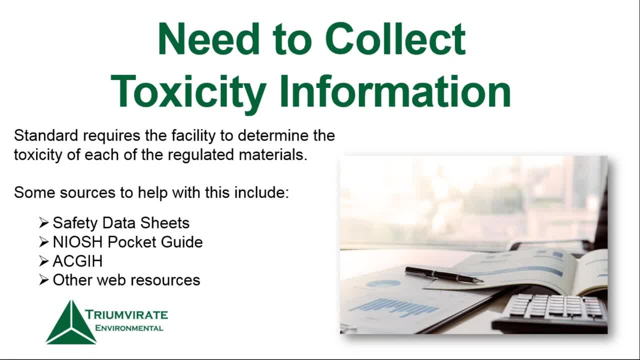 didn't have a lot of the data resources that we have today. and I always say to everybody to I always caution, I always caution, caution, caution, because you know it's like, you know there is other web sources out there, but remember, where are you getting that information from? who is who put that information out there to 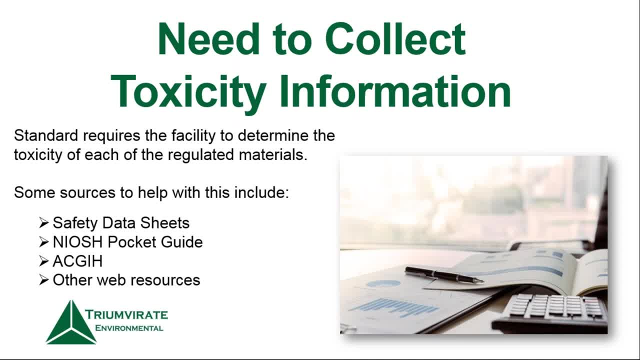 make sure the accuracy of it. so I strongly not recommend here that you use things like the safety data sheets that you always already have. most years may be familiar with an iosh pocket guy. you know hazardous chemicals. that's a great one. a CGI h, the American Conference of 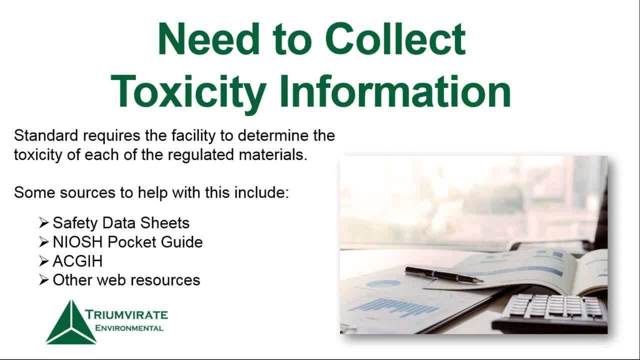 governmental, industrial hygienists- somebody say that ten times fast. and also there's plenty of other web resources out there. you get toxnet, you got you know so many other different outlets out there that you can meet, you know, you can look at and refer to, to collect data, to. 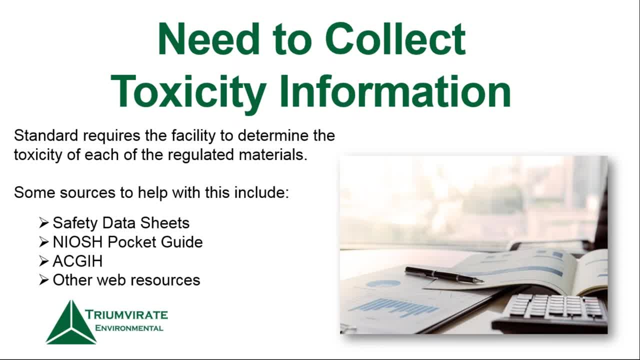 on some of this stuff that you may or may not be as familiar with, but you want to be familiar with because that's going to help you to figure out. all right, am I in this program or am I not in the program? and then figuring out, all right. 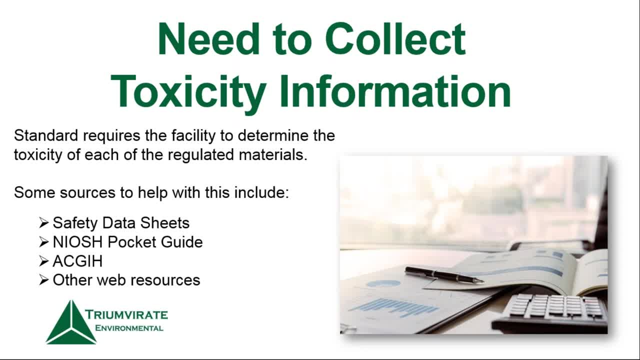 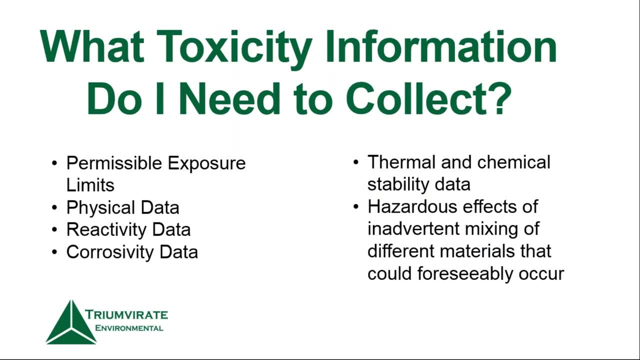 what do I need to do to ensure that nothing really bad happens as you go down the road here? so what type of information do you collect on all of these chemicals? again I want to stress: these are for your regulated chemicals. so if you find out that you have more than one regulated chemical, then you 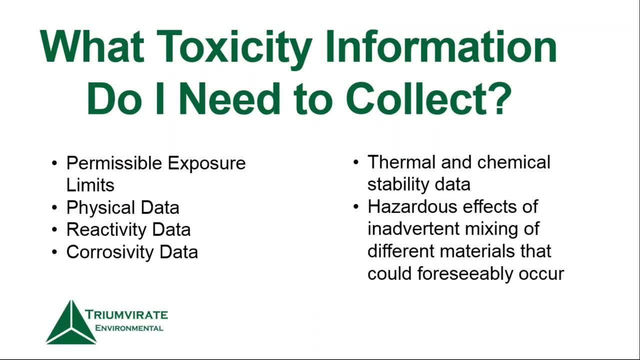 want to do this, even though I would suggest a baby. you do it, for you know anything that you have that's even close to being, you know, the threshold quantity or the TQ is. it's never a bad idea to look at that also and say, hey, at least. 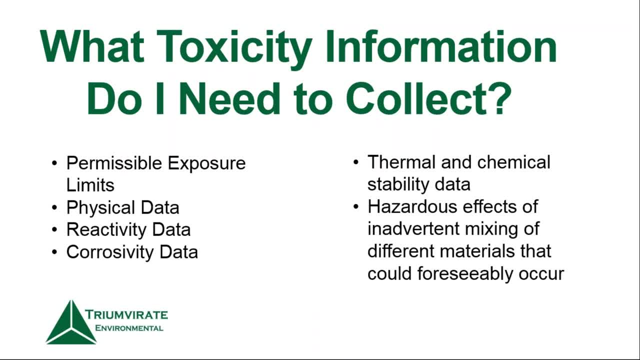 I'm collecting that data because you know what if tomorrow we change a process and now we're over on that material? at least you've already done all of the homework. so, as you can see on this slide here, you can see that you've already done all of the homework. so, as you can see on 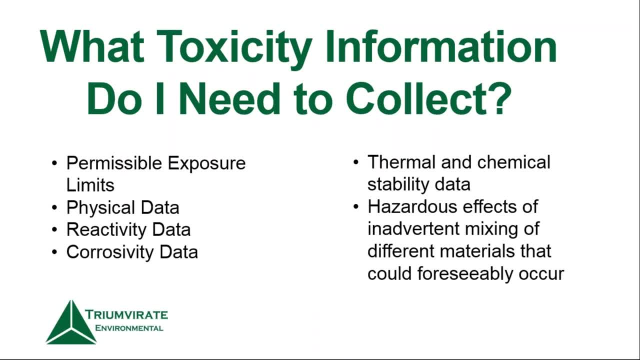 this slide here. you know we want to know about permissible exposure limits, your physical data, your reactivity, corrosivity. you know you kind of understand. you know what- a- most importantly I think, is the last one here- what happens? do you have any of these materials that could react violently? 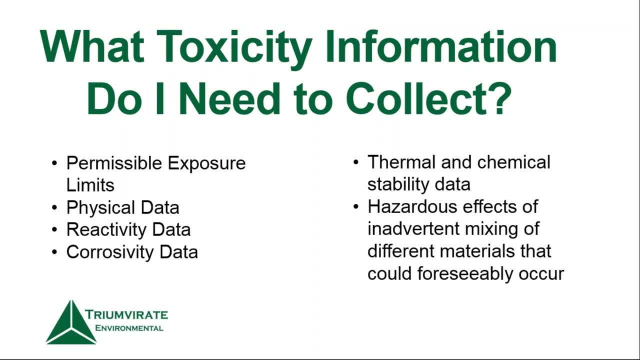 with the other material that's regulated. so you want to be looking at also any types of incompatibility issues that you have at your facility and then kind of play out because this is a lot of what-ifs, it is a lot of that doomsday scenarios. as I always say to people, I try not to 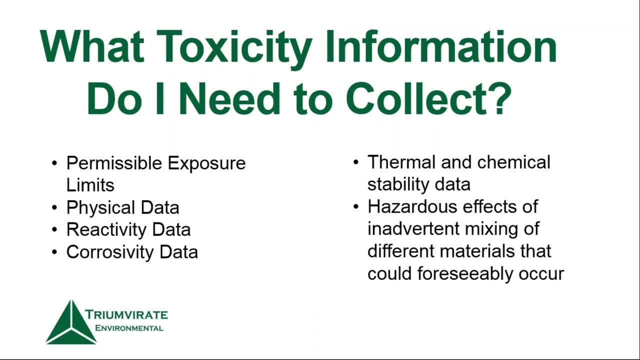 be the doomsday. you know preacher here that, oh my god, the world's gonna end tomorrow. but there is times where, in this case here, we do need to look at that, because these are the things that we are trying to prevent at all costs. if we absolutely can, that is what we would like to do, so that's a major part of all. 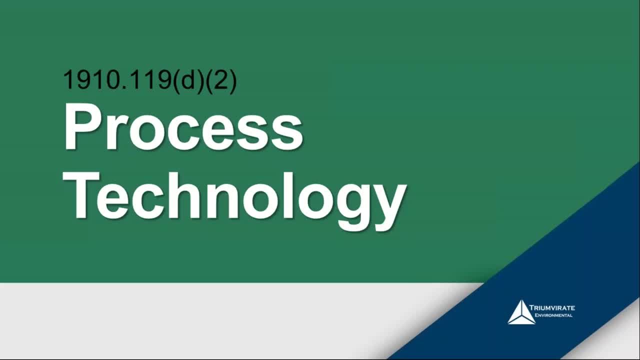 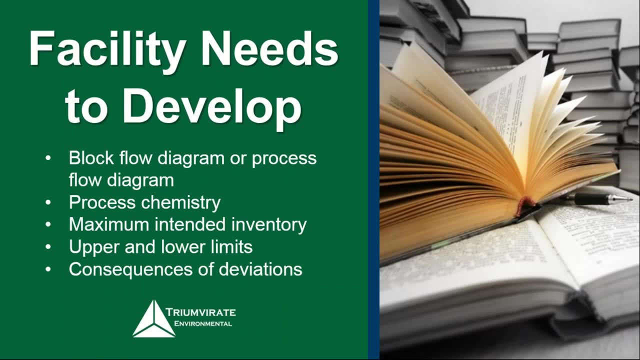 of this is collecting this toxicity data from there. we're going to look at all the process, right? you know what do we got for technology on how we do this. so what do we mean by this, or what does OSHA mean by this? right is, they say, the facility. 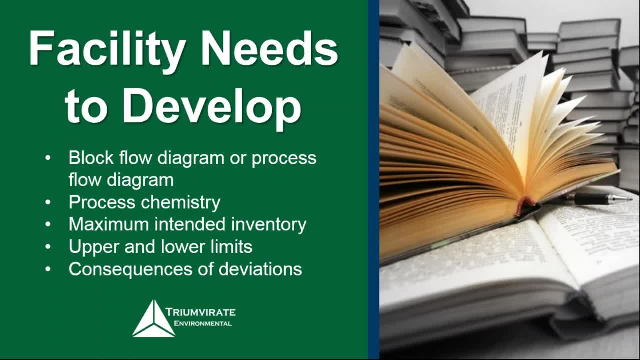 needs to develop. as I already mentioned this, you know it's kind of a block flow diagram, process flow diagram, whatever words you want to use. that really traces how this material goes through the facility. how does it work, where does it go? how does it? you know what is the dangers. is there potential in there? my 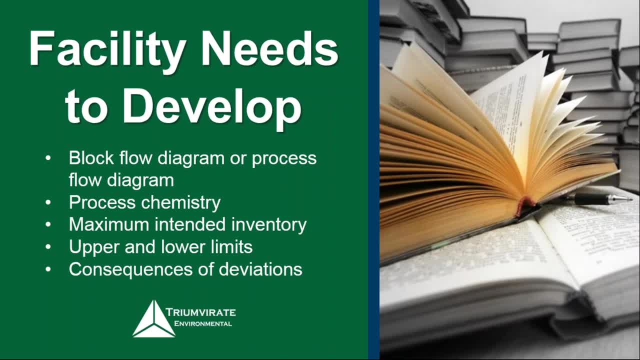 favorite word is potential, right? is there any potential of this stuff coming in contact with something that it doesn't like? and you know, really fearing all of that. Oh, plus knowing, okay, you know. do you have any controls on how much of an inventory you're gonna have of these materials? you? 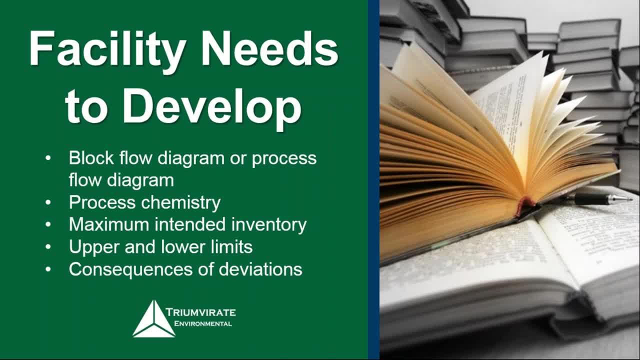 know sometimes- and I had a client once that was getting close on this- and they're like: no, no, no, we're gonna make sure that we don't come. you know, we're just under the- you know the threshold quantity for the chemicals, so that we make sure that we're not going over it. and then they realize that they could be. 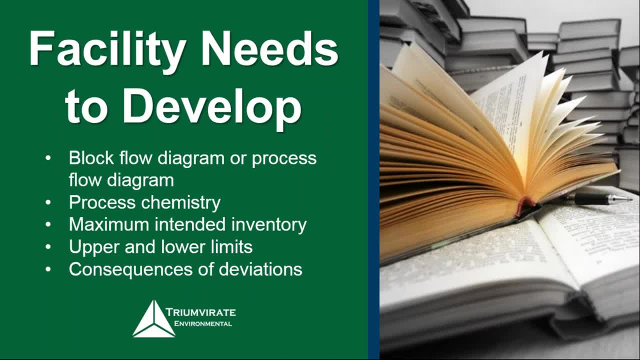 cut it back even more substantial than that. so that's stuff that you want to look at, and then figuring out: what are the upper and lower limits of that, how much do you normally have, or how much can you have less of, or anything along those lines, and then also, what are you going to do if you exceed any of this. 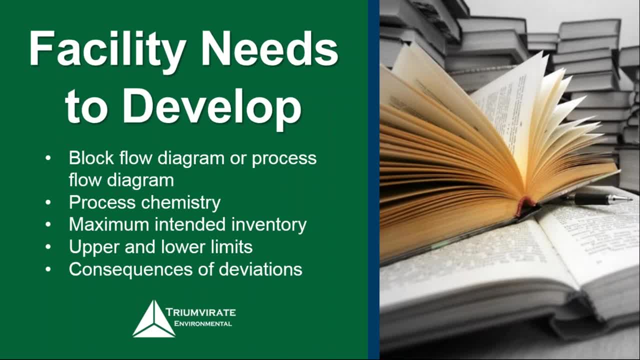 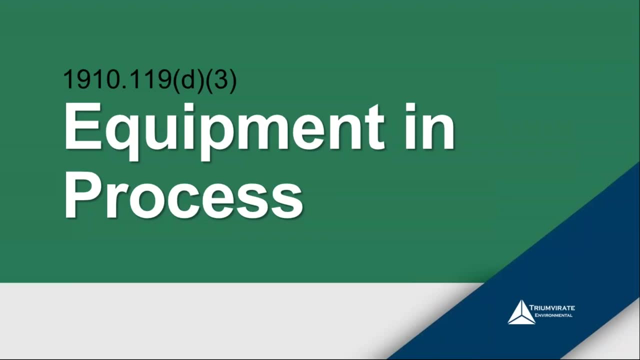 stuff or you deviate from anything you said, you're going to do so again. it is doing that, pre-planning out and saying, okay, I need to do this, I need to do that, I need to figure out how to, you know, move around in this program. so already you can probably see that, wow, there's a. 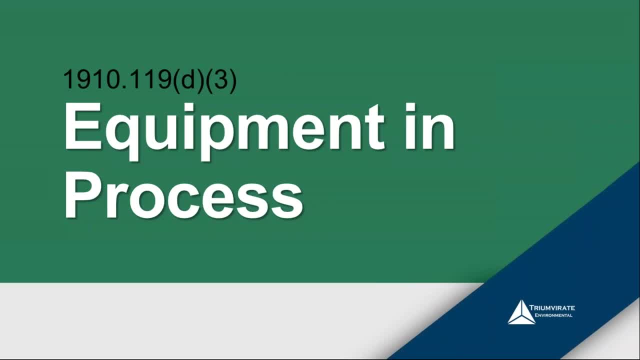 lot of little things that I have to do, and it truly is. there's a lot of stuff within this process, so some of these next few slides I'm going to go through relatively quickly, just based on time. but you know like you also have to look at all the equipment that's in the process. this can be, in my opinion, this: 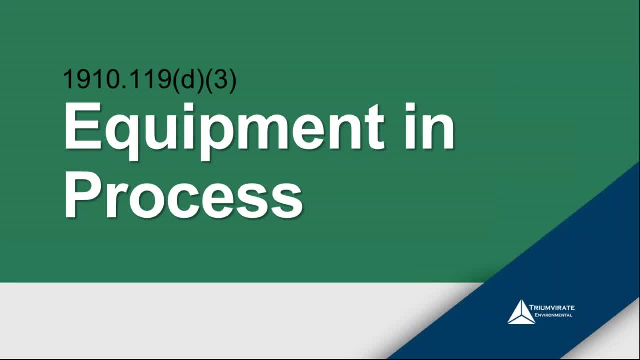 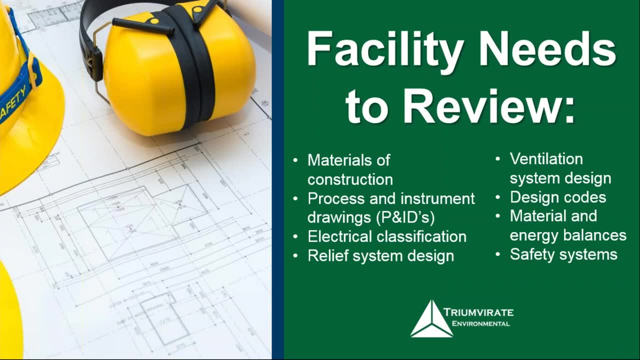 can be sometimes the hardest part of it all because you may not have any of this data or it might be harder to find because you're at up, you know an older facility, so sometimes the older facilities have you know you may not have all of this data ready available, kind of like you know what's, the materials, the 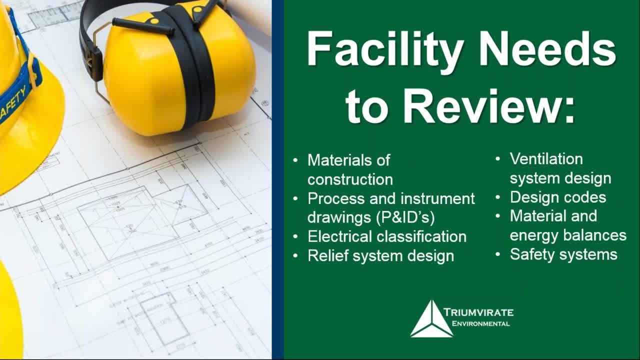 construction of it. you might be able to guess, but you may not have it, you know. do you have any? what types of drawings do you have? you know the electrical classifications. what relief system designs do you have in place? how do you do that? what about the ventilation? and what codes did it follow when it was? 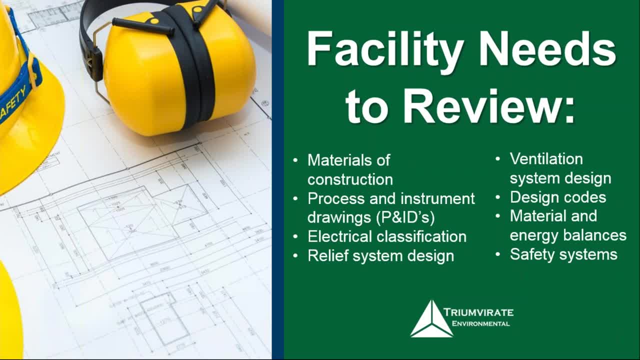 being done, you know, and what types of safety systems. some, like I said, some of the older stuff that we look at is not as safe as things are today. they don't have all of the quote-unquote safety features, so it can get a little bit more. 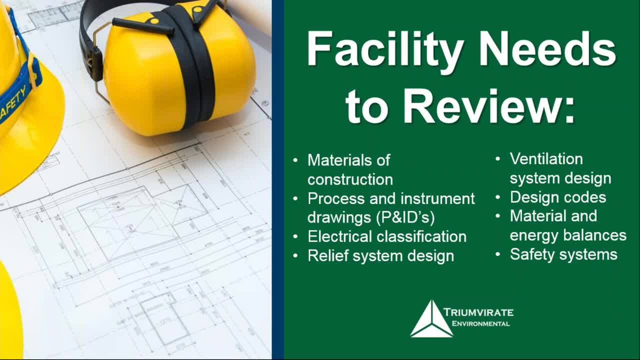 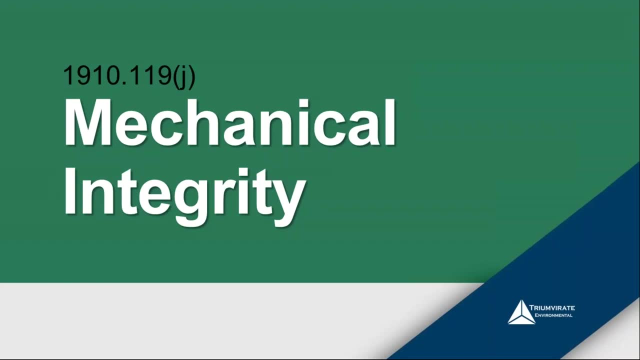 difficult for you to be able to, you know, figure out all of this information, but it's an integral part of the process that you must do this to ensure that you collected all the right information. then you have to look at, you know, the mechanical integrity of the equipment that you just looked at. so what do we? 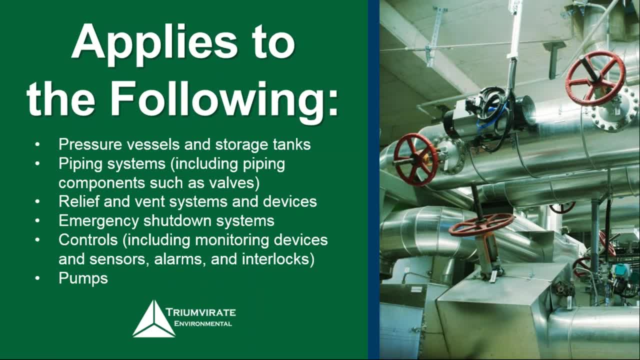 mean by that. it applies to certain pieces of equipment that we were just reviewing. so now we made a list of all of the materials that you know, I'm sorry, all of the machinery that's involved. but now we're going to look at it and say, okay, do we have or any of these instruments here? part of that you know. 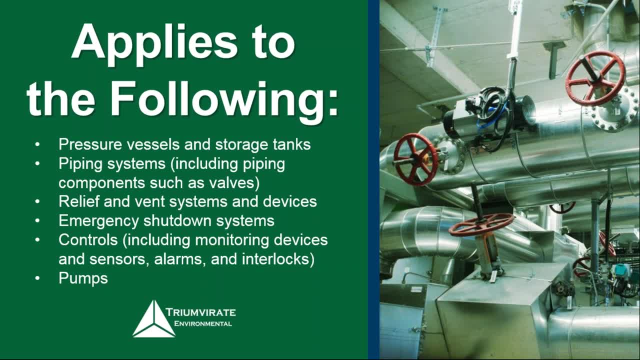 especially here, like pressure vessels and storage tanks. right, if we're going to do a doomsday scenario, probably the first thing we want to do is have a tank explode. right is because that is the worst case scenario. so that's why they're looking at those. and then what? 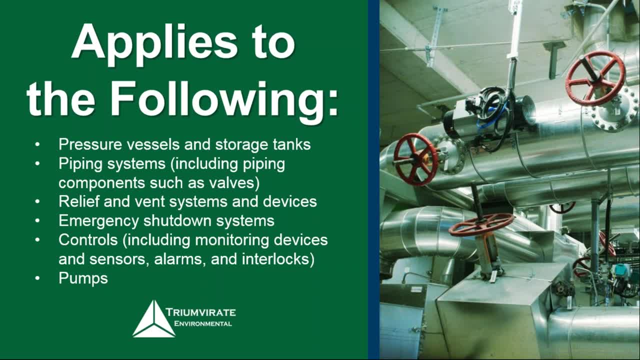 about the piping systems right. most times it's not a problem with the tank itself is historically, if you look back, and even the chemical safety board or anything like that, when they look into incidences they always say, oh, what usually it is is what more of a piping or a valve release or something like. 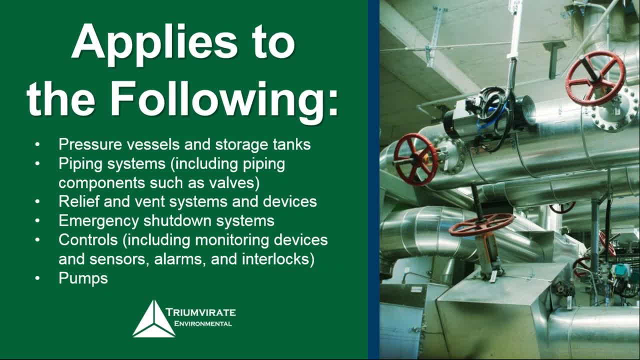 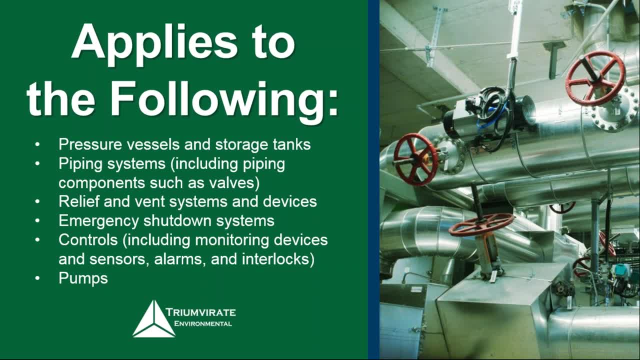 like that. so that is some of the things that you really, really want to look at, and when you're doing that, you want to make sure you're looking at. you know the shutdown systems and they work. are all the controls? how old are they? how many was the last time you tested them? things like that is because that's all very. 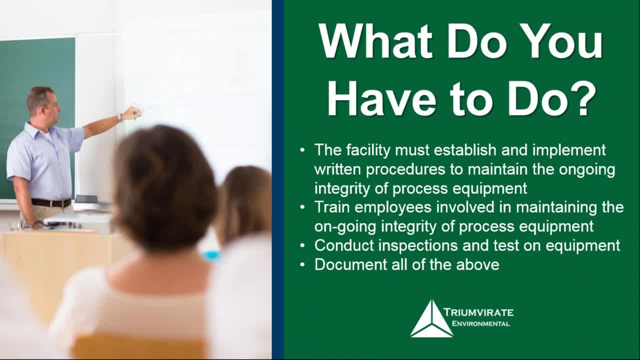 very, very important to know and how to maintain those. so what did they make you do after that? so once we figured out, alright, where all this stuff is in the program, So how are we going to maintain that? So how are we going to make sure that you know that Joe Welder is, you know? 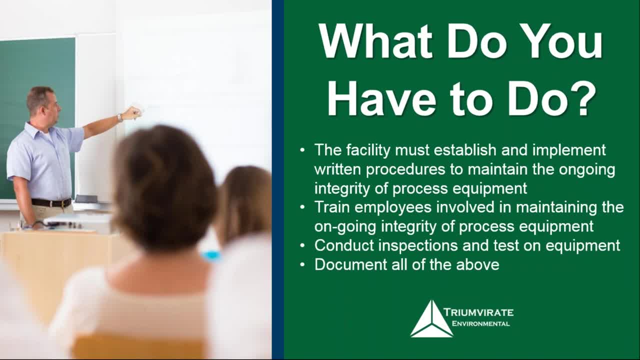 hey, or you know, you've got a structural engineer that says, hey, I'm going to change this because I think that in the process we can change the way the piping goes. Well, that could have, you know, a very strong problem. 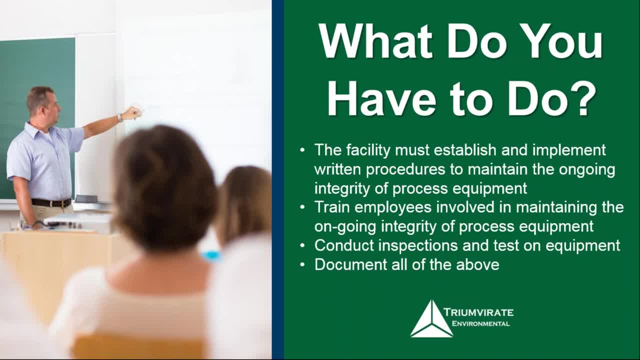 or cause a problem in the process. So therefore, you want to make sure that that's well documented, Because you've also got to train all your employees- you know that are maintaining this equipment- about what they can and cannot do. So then, from there, you've got to make sure you're conducting inspections. 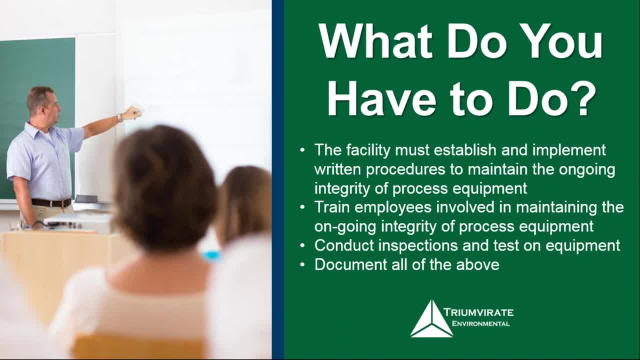 And we'll talk about that a little later. But inspections is a huge part of all of this too is to make sure you know if any of you are ISO. I say this is very similar to an ISO process plan: do check, act. where you're planning it, you're doing it. 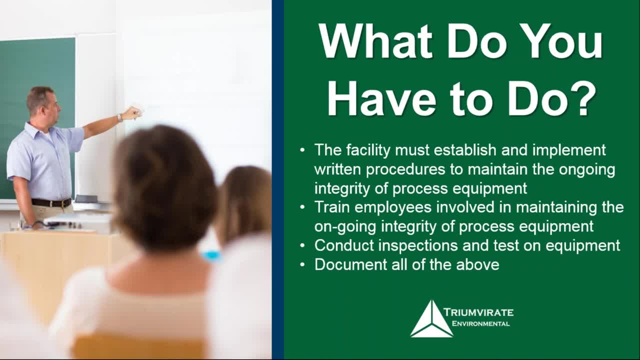 you're checking it and if something's wrong you've got to act on it. Once you get back to there, you're going right back to the start of the process again, too right, And saying now I've got to start the planning process again. 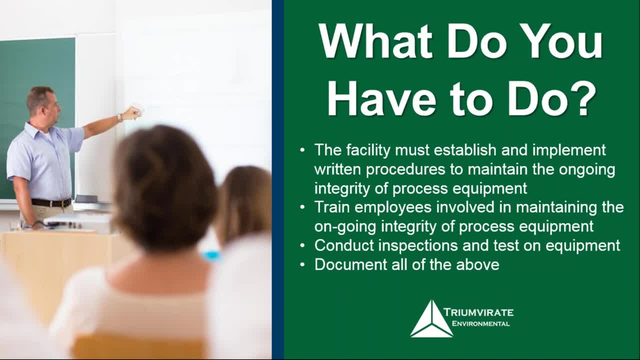 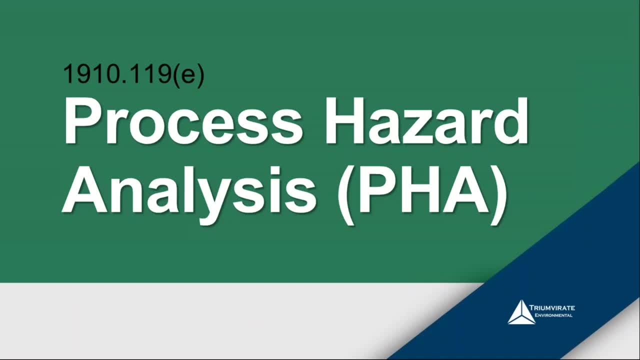 and I've got to keep going around, around and around in a circle just to make sure that I'm constantly meeting all of the requirements. All right, PHAs- you know this terminology is thrown out there a lot today. I hear this term a lot for different entities. you know of work. 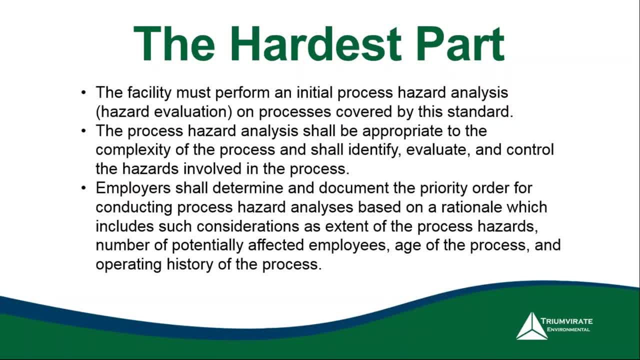 But in my opinion, this is truly the hardest part of this entire process. okay, Because we've already figured out all right. now we know: all right, are we in the program? Unfortunately, we couldn't get out of it, right. 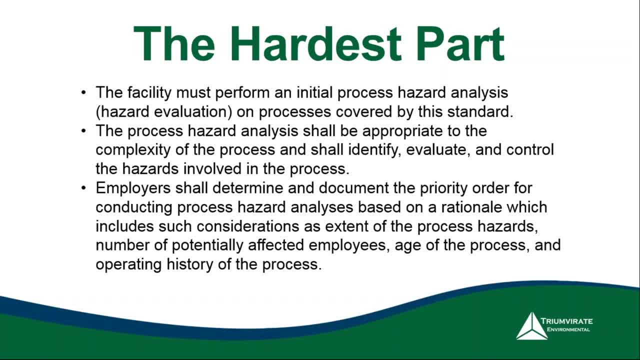 From there we started putting together our process flow diagrams about how the materials flow through the facility. We've looked at the machinery that we got part of it. We looked at the integrity of that machinery. But now we've got to figure out and say, okay, what could happen? okay, 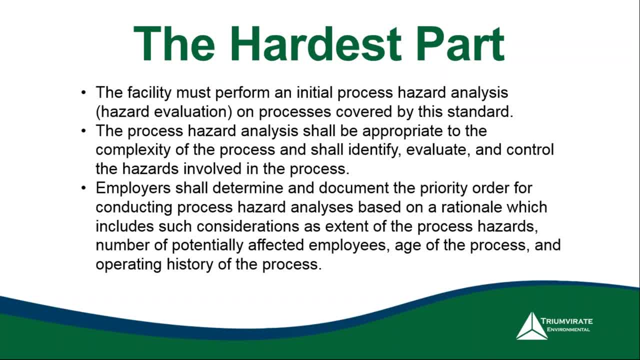 And these: I cut and pasted this right out of the regulations because I thought it was the best way, you know, to kind of really lay this out. So the first thing that we had to do- and I think this is a really interesting point- 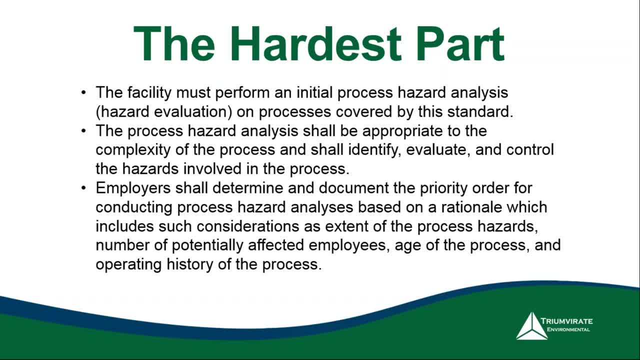 is. it says here that you have to do an initial hazard evaluation on all processes. Okay, but look at the way they word this. The process hazard analysis shall be appropriate to the complexity of the process. So they understand. OSHA didn't turn around here and say to you you must do this this way. 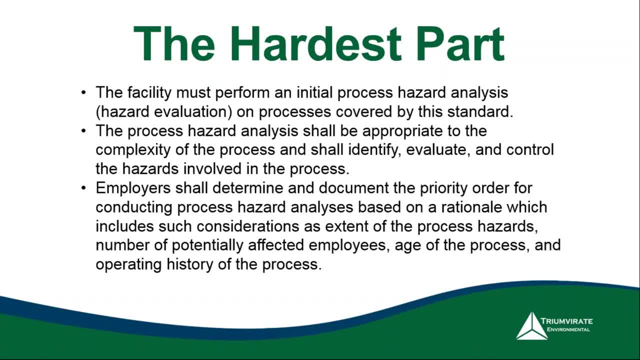 They said, okay, you've got to be as complex as the process itself. So that always makes me a little bit nervous, because that's very subjective, right? Because that can be very subjective on the person that's evaluating what you're doing. 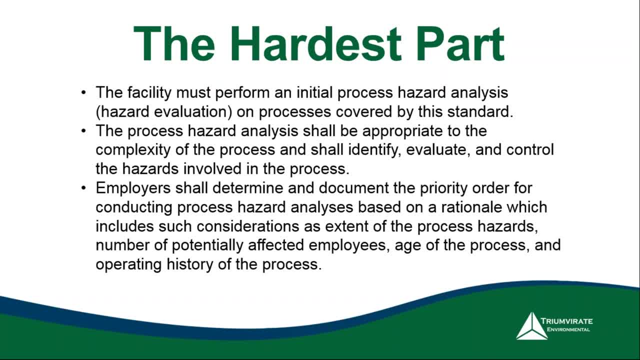 and how you're doing it. So back to that documentation piece is I always say: you really, really, really want to document. well, why did you go the route that you went? What was the justification? Back to our committee earlier. 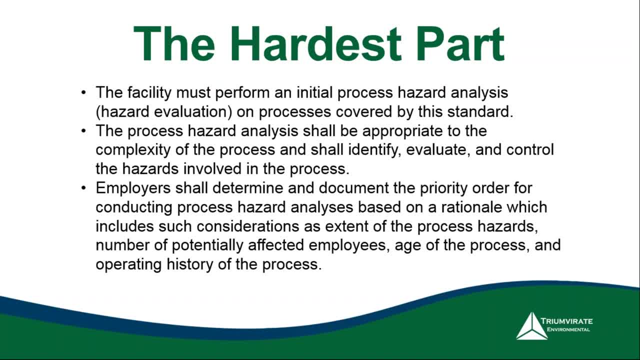 Put it out in front of the committee and say: all right, how you know complex, do we need to go? Is this really really detailed or can we make it a little more simpler? Again, document every part of that, because 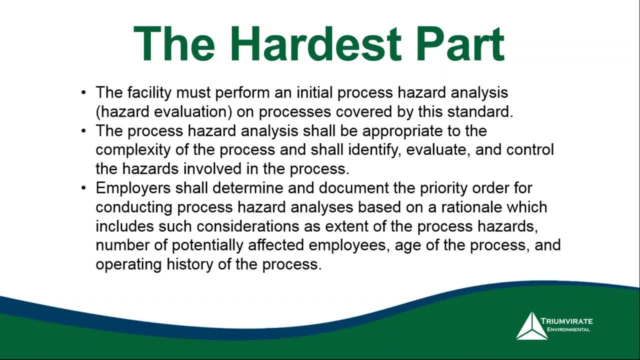 it will help you in the process as you go along And keep into consideration all of these things right. How many people are going to be affected? Who's going to be affected in the surrounding areas? Things like that are all an integral part, okay. 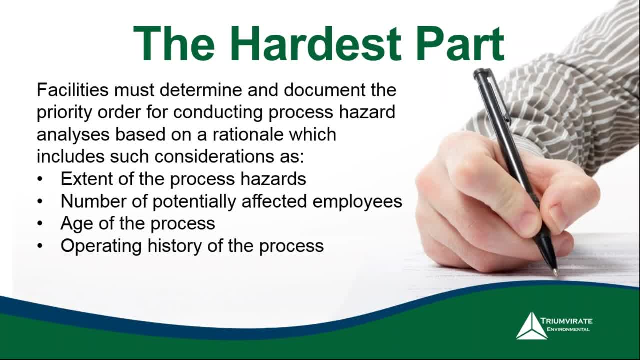 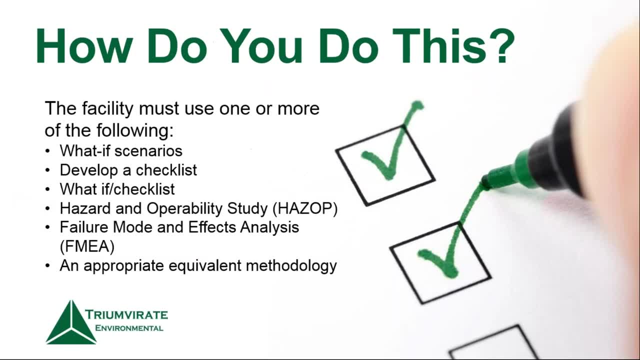 Then from there, you've got to determine and document and prioritize: how are you going to do this? okay, How much are you going to do, How are we going to do it And why are we going to do it. And then from there is: how do you do this? 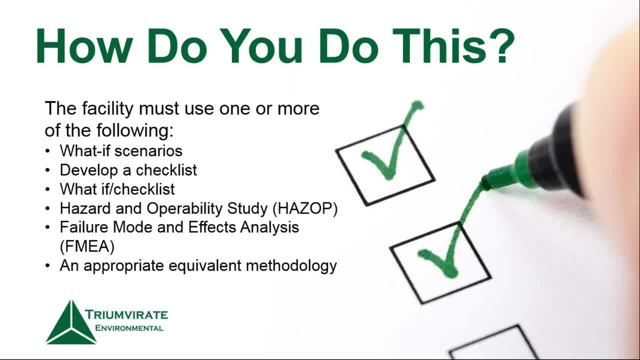 Well, OSHA says you have to. You have to follow one or more of the following, which is: you know, you do those what-if scenarios, So what if that tank ruptured? But you know, when you're looking at the what-ifs too, it's not just saying: okay, well, what if it did? 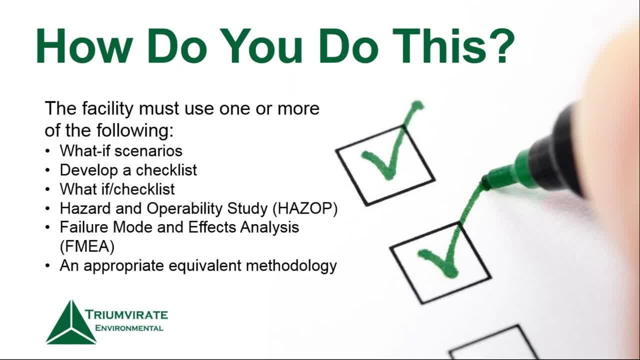 You know when did it do it? Is it in the middle of the day, in the middle of the night, or you know, is it on a weekend? Or you know what, if it was at a you know a peak time, or when can it go? 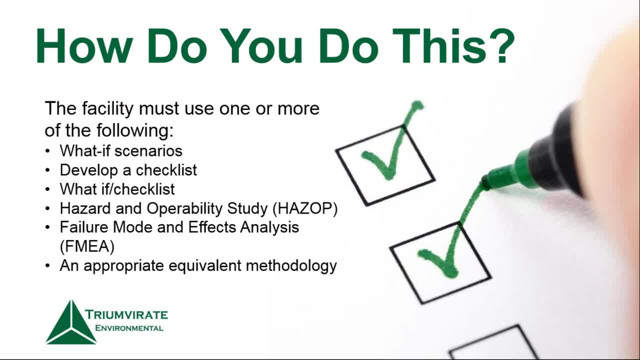 Things like that. They also. you know, you can just develop a checklist to say, okay, we've analyzed all of these different types of steps in the what-if scenarios. That's why we have the what-if slash checklist. Okay, You can do a HAZOP is what are we doing? 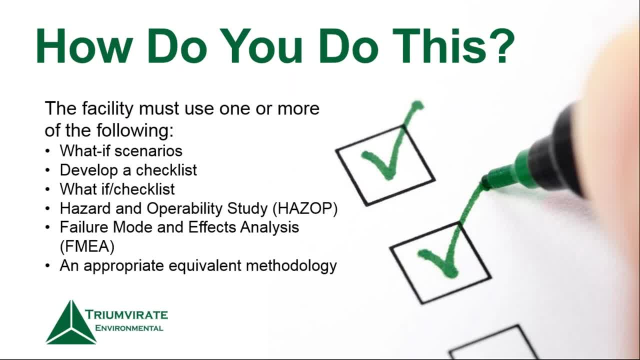 You know what are the hazards, and then what is the operability, How do we do that? And then the failure mode and effects analysis, which is one I've done. is said: okay, hey, you know, if this did fail, what are the effects of that? 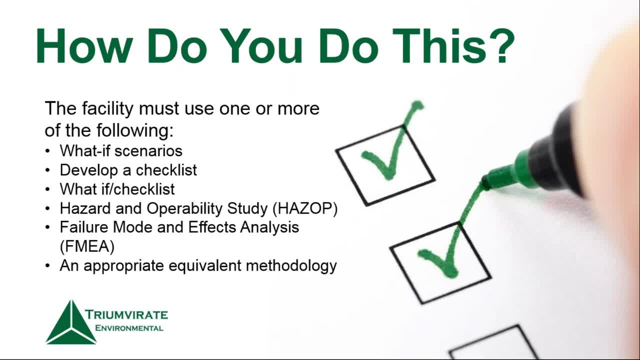 So sometimes it could be doing some type of dispersion modeling, depending on the complexity of your facility Is you might have to do, you know, some type of like cameo or aloha or any of those you know types of a data check, to say. 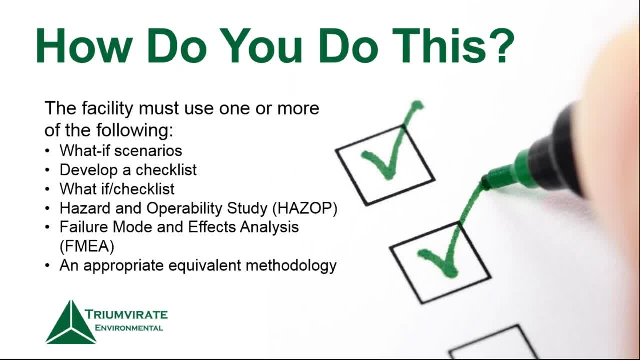 ooh, okay, if that pipe ruptured and this happened- and where did it happen? is that we might have a plume cloud that could go here? Well, that's part of your scenarios and you've got to figure it out and say, ooh, okay, we might have a problem here. 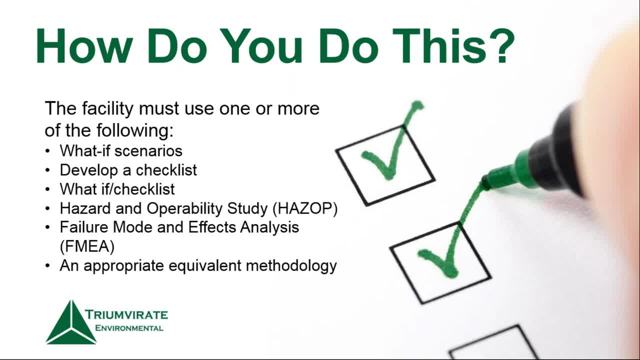 You know danger, Will Robinson type of a you know scenario that you want to worry about, And you know it also gives you the out right, It says an appropriate equivalent methodology. So again, if you can sit there and justify and say, okay, you know, this is what I want to do, you know, and this is why I want to do it. 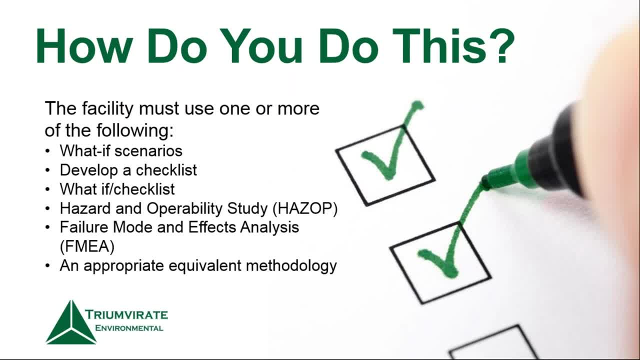 and this is, you know, all of the different scenarios that we analyzed. that's fantastic. That's exactly what we, you know. what we want to do is to, you know, make sure that we've documented every single part of this so that we didn't miss something. 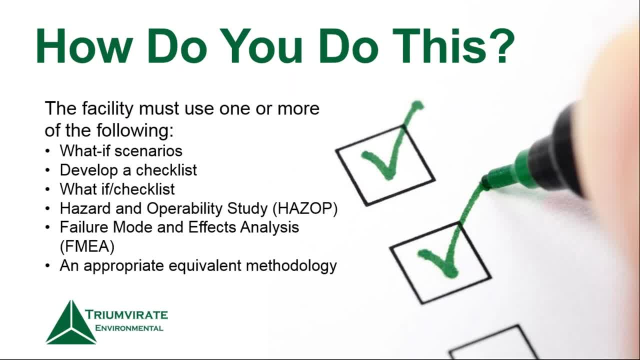 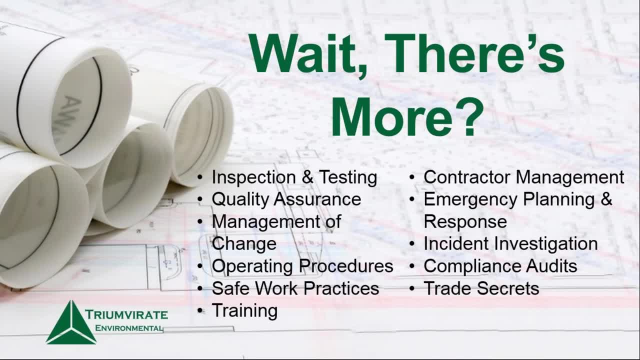 So you know you really want to document, document, document. You're not going to hear me say that enough, but it is a big part of it. Okay, So don't worry. kind of like those infomercials, right. 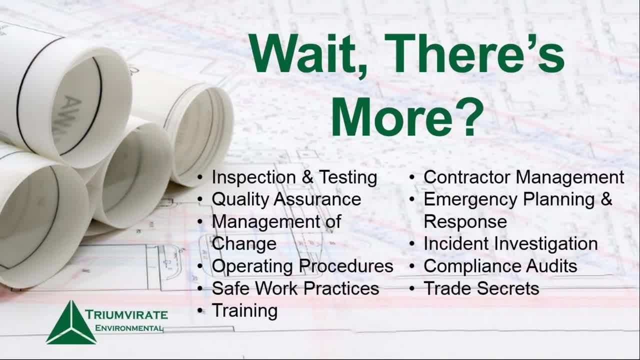 Here's those infomercials for you. You know, wait, there's more. If you order today, today's free is. you know well, it isn't quite that way. But okay, there's all of these pieces here, come with it too. 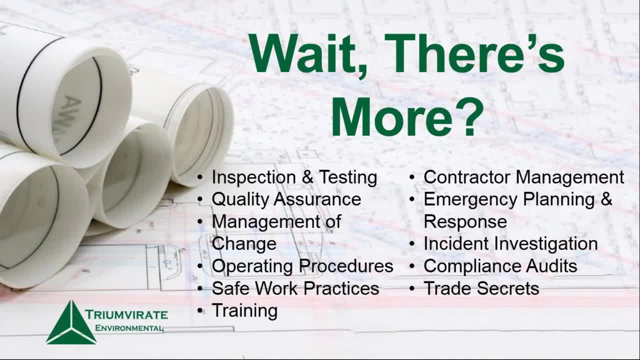 And, like I said, I'm going to you know we're going to briefly go over some of this stuff, but I think it's very, very important that I want you to understand that there is there's a lot of pieces to this. 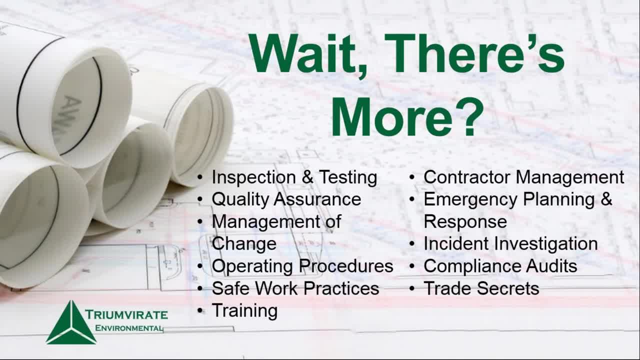 And of course we have to say it right, There's got to be training, safe work practices, emergency planning and response. What are you going to do? Do you have a spill response team? How many of you that do have a spill response team and then find out that you're in the process? 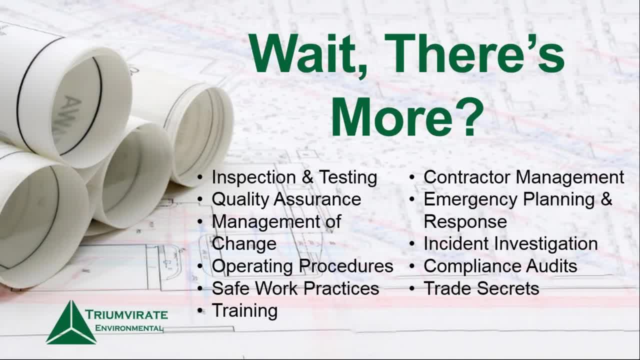 safety management program have actually taught your team, your hazmat team, about your PSM program, Because the two are interconnected and they should be. So that is something, too, that you know. when you look at these programs, you say: 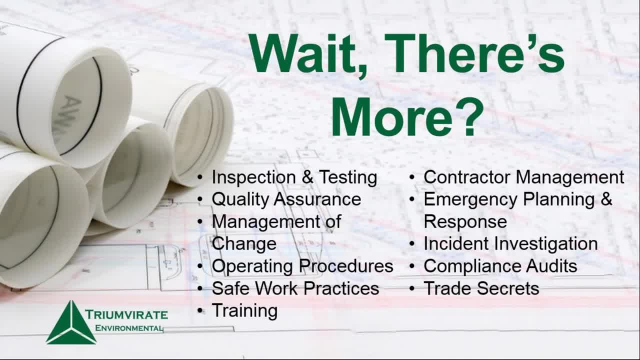 well, how come that wasn't mentioned in the training? You know that you had this program or plan in place, So it is something you know to think about. But let's just quickly go through some of these. Like I said, I can't, you know, we just don't have the time to go through every one of them. 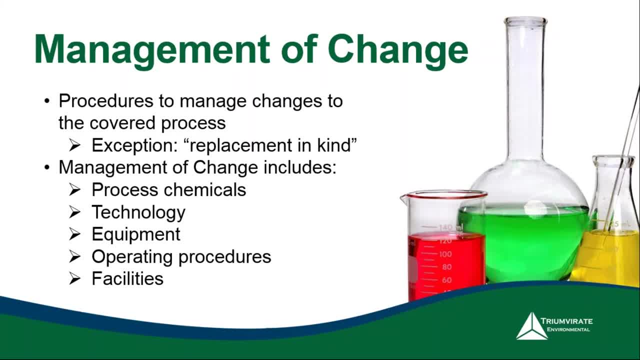 So I did pick and choose just certain ones that I thought were important, which is, you know, it's a lot MOCs, as some people call them. right is the management of change, And this is to say how do we do it. 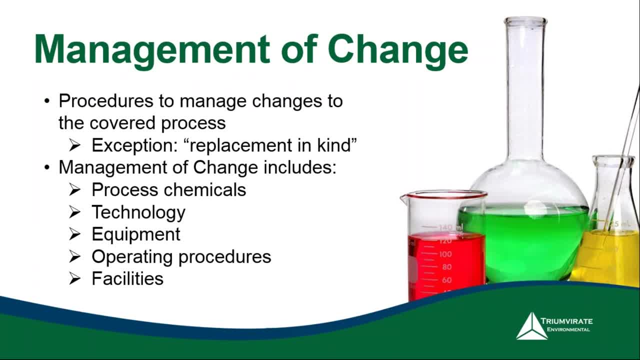 You know what. if we change something, You know how do we change it. What do we have to, you know? is it a process, chemical? Is it a technology? Is it the equipment? Did we upgrade some of the procedures, the operating procedures? 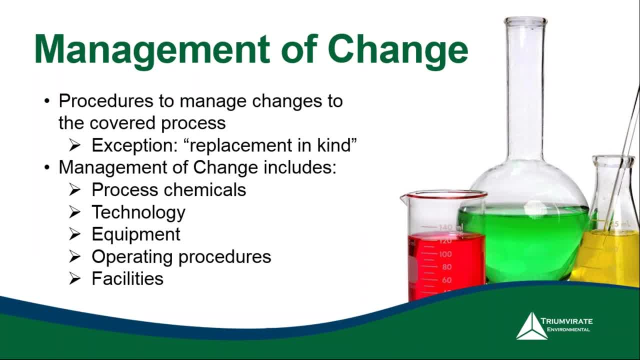 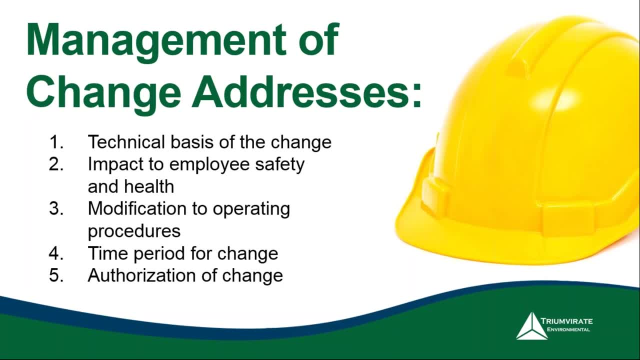 Did we change something at the facility that could have affected this program? Because if we did, we got to do something about it. okay, And then what do we? got to do, We got to document all of that right, And to say, okay, what was our technical basis for that change? 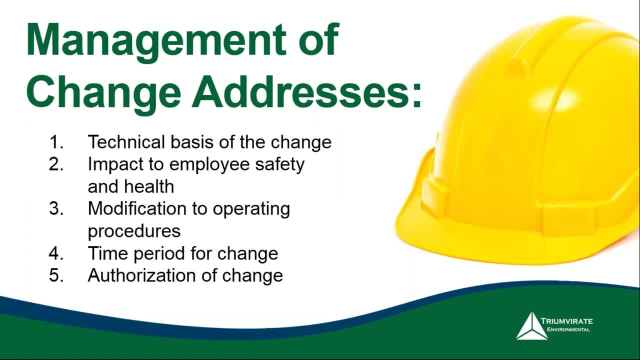 And it wasn't that. you know, John slept at a Holiday Inn last night and now he feels like he's a chemical engineer. So we really want to make sure that you know you're looking at everything. What is that impact? right? 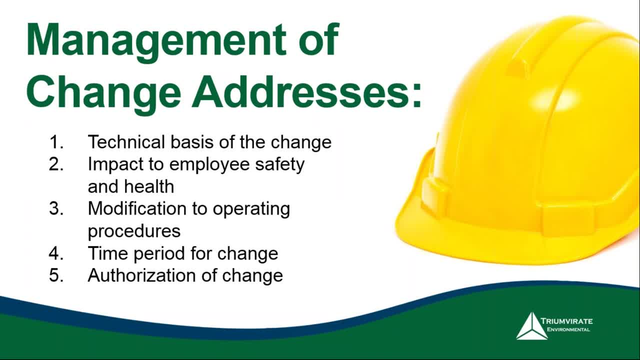 What is the impact to everybody involved with this? Was there an impact? Is it a good impact or a bad impact? Did you have to change PPE? Did you have to change? you know anything else? Did you you know when are you going to do this? 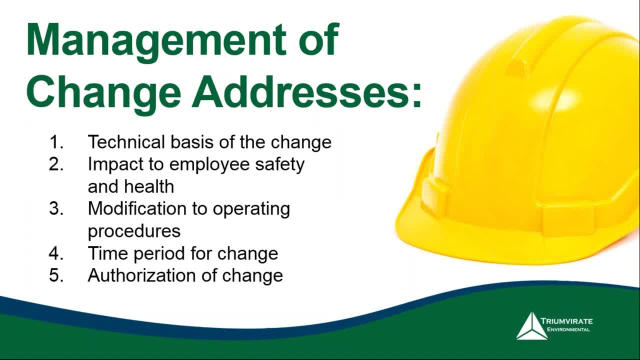 Did you have the paperwork trail? Remember we said document control earlier on? also, Did you have that authorization here of change to say, okay, this is how we did it, This is why we did it And that, yes, you know whoever we authorized to sign off on it has signed off on it and ensured that things are correct? 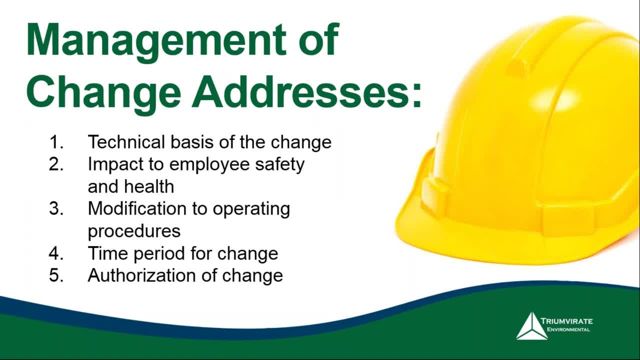 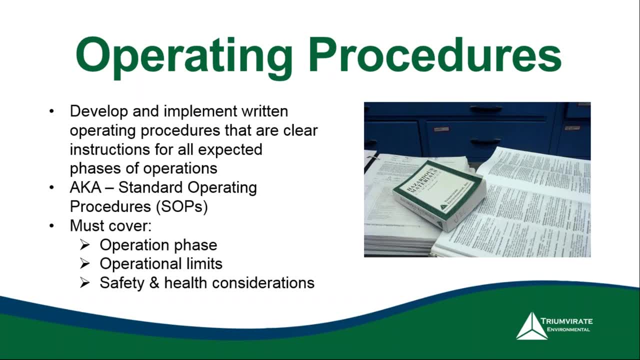 So it is kind of a process here that you need to go through in order to make sure that everything is correct. You've got to have the operating procedures right And again, this is, you know, their words, not mine- right. 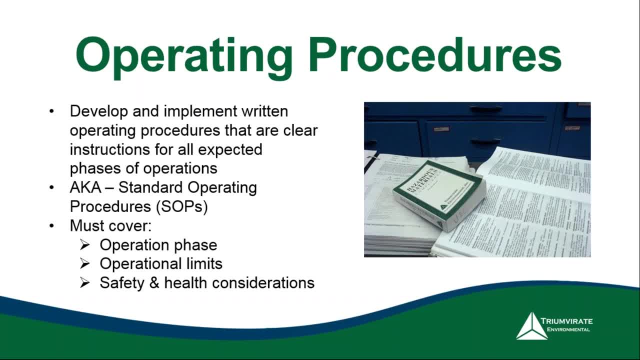 It clearly says there are clear instructions- clear. I don't know about you guys, but you know, sometimes when you get instructions you just sit there and you go what And typically right- like at Christmas time when you get the instructions how to put something together- most of us don't look at them, right. 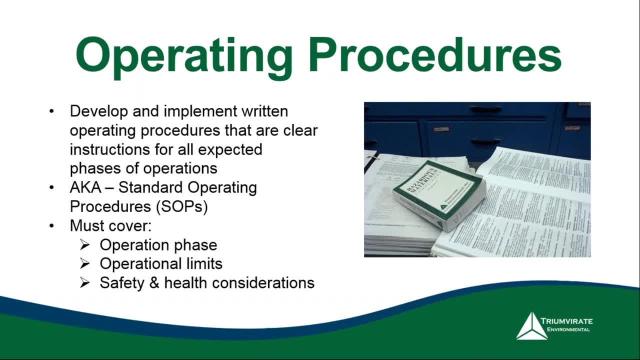 So you really want to make sure- This is where I say you want- to get your employees involved, people that are actually going to do it- Put it in their language, Put it in this you know know-how so that they understand it. 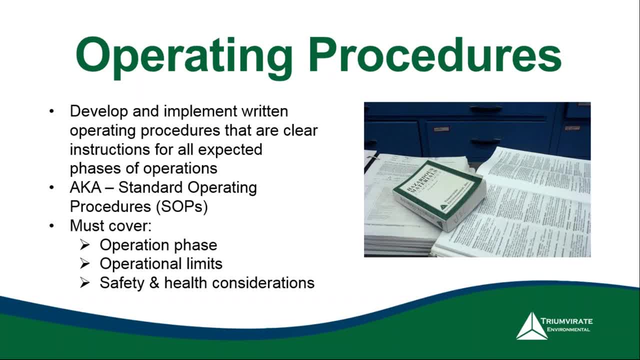 Because who's going to be looking at it? the most Them And you know- and then just make sure it meets all of the requirements you know of what needs to be done, like it says here. You know what are we doing. 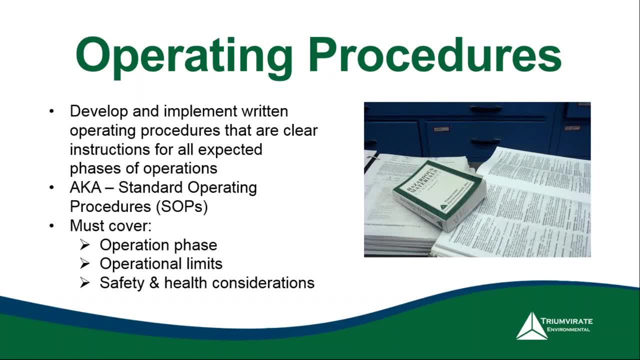 What are the limits? What did you look at for, you know, for safety and health considerations, Because, again, all the way through this right, what's our number one concern Is the safety and health of our employees, or anybody that's in those areas. 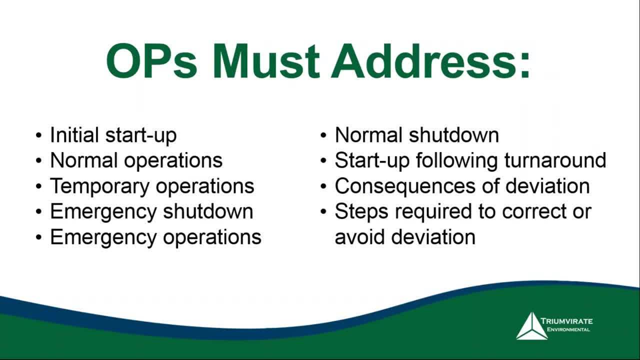 Because, God forbid, something was to go wrong. So all of your, you know, the operating procedures have to cover all of this at a minimum. okay, Everything from the initial startup to normal, to temporary, to emergency shutdown. You know, I've seen emergency shutdowns too, where people say, oh, I hit this button. 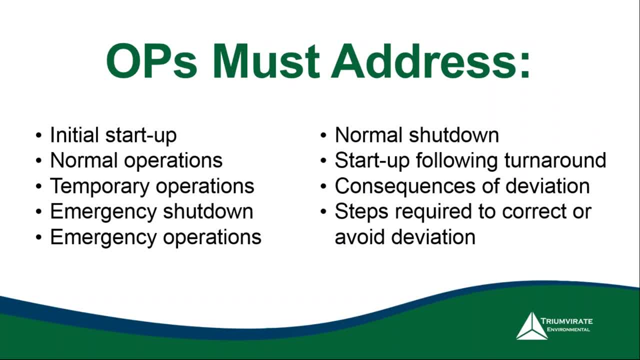 And I go, all right, did that close every valve, every electrical outlet, everything that could potentially go in there and control temperature, Or is it pressure Or whatever? You really got to get into that detail Again. what are you going to do in case of an emergency? 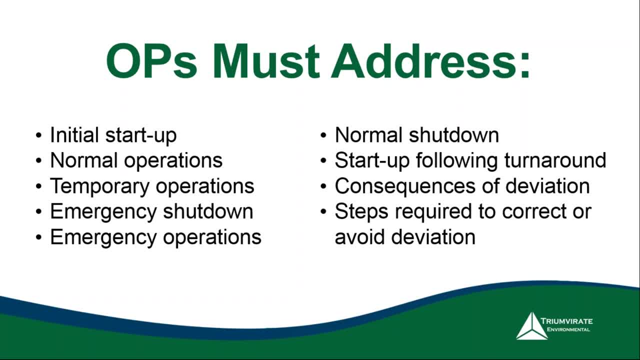 How are you going to do startup again? What happens if something didn't go right? Back to your, you know, back to the earlier hazard analysis, your process, hazard analysis. it's going to tell you how do we do things. okay. 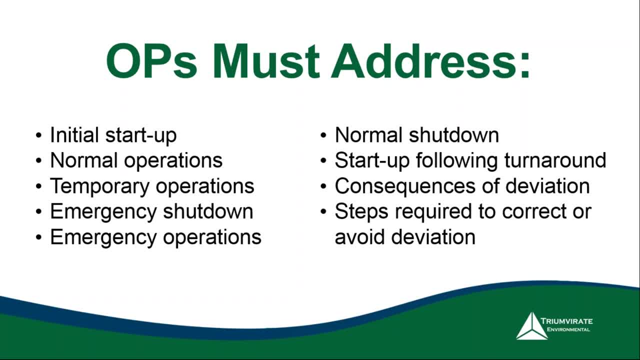 And then, what are you going to do if you had to correct, or how do we avoid a deviation? So what safety devices did you put in place to make sure that some of this stuff would never happen? Because that's really the key here is to say to yourself: okay, I've got to make sure that you know, this can't happen. 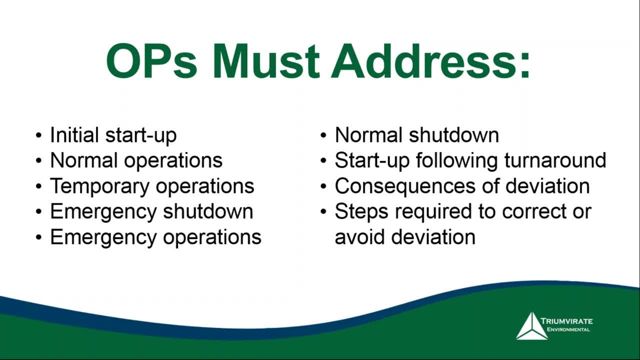 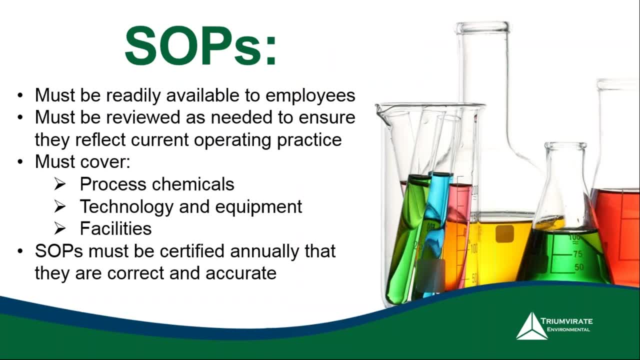 And we've got to do our best to make sure that it can't happen, And we will, you know, go from there All right. So then you've got your standard operating procedure Again. more of them, right? Look, they've got a very similar to our safety data sheet, right? 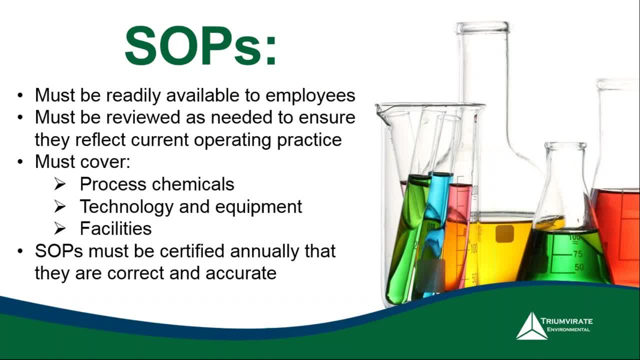 They've got to be ready, available for your employees to see, They've got to be reviewed to make sure they are current. So, you know, I typically like to say, hey, you know, an annual, you know thing is great. 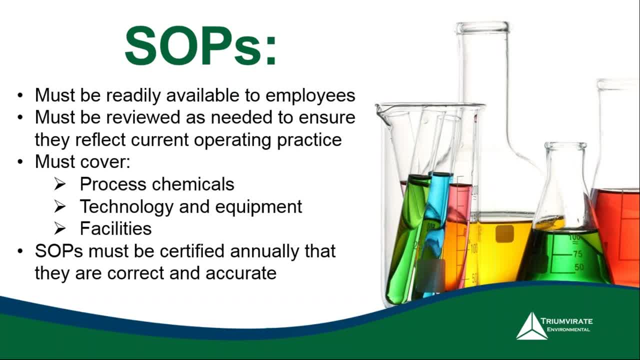 But sometimes depending- again back to remember what I said earlier on the PHAs was depends on the complexity. So at a minimum you're going to do it annually, right, But maybe in your facility it might be every six months- makes more sense is to do that so that you, you know, know that you have it correct. 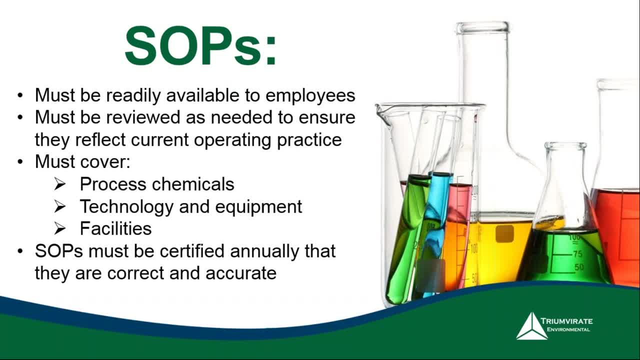 And you know if you're a chop shop, as I like to call it, right, you know, if you're somebody that's constantly changing processes, you know you're making different products for different clients. well, that may mean that you've got to look at these on a more regular basis than just annually. 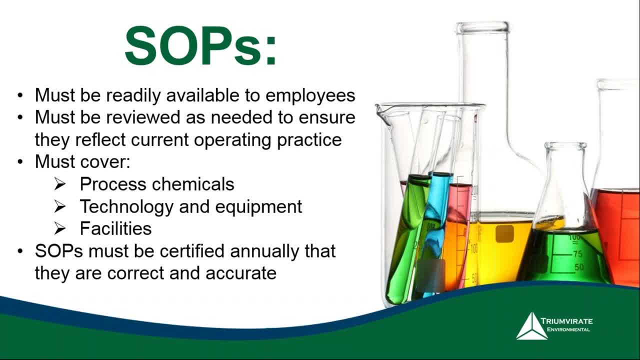 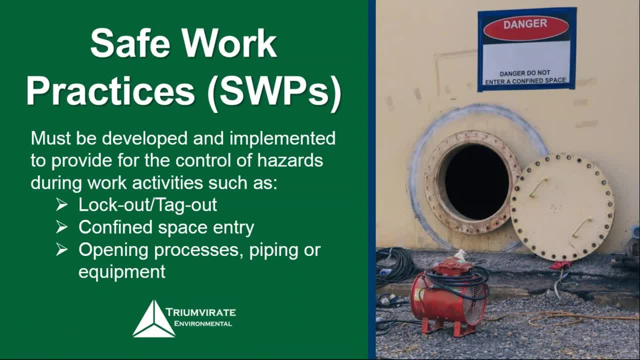 So it is something that you want to take into consideration as you are going through this process Again. so then you've got to have safe work practices, right? This is again, how do you do it, And this is where this rule will stretch out into other regulations. 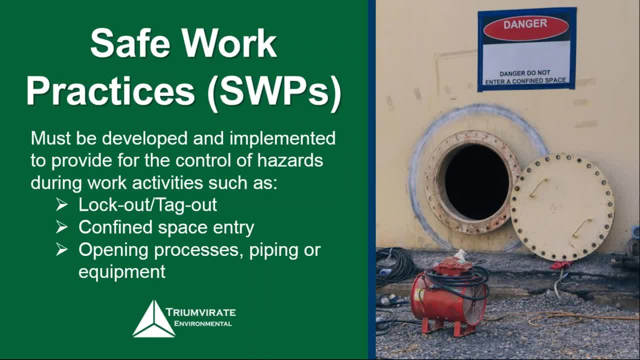 You know, you've got to be aware of right, Because part of our PHAs and part of keeping people safe might be that we've got to lock out or tag something out. We might have to do a confined space entry. So then we get into what. 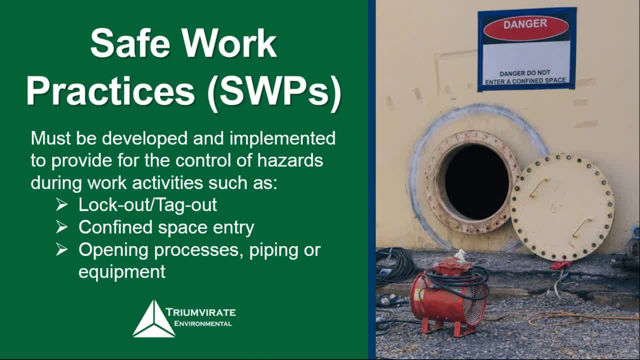 Personal protective equipment too. We have. you know you might get into welding, cutting and brazing. You might get into, you know, hazardous chemical rules. You're definitely going to get into HAZCOM. So your HAZCOM program should also have some illusion. I'm sorry, some direction. 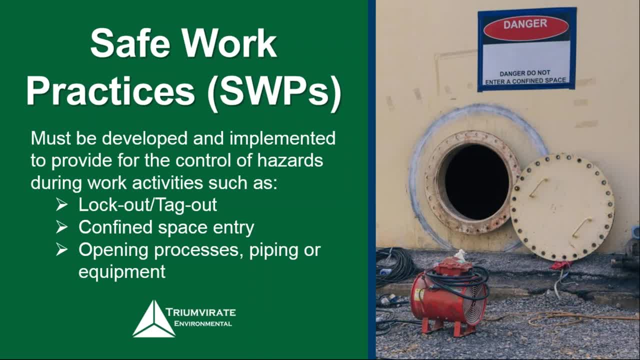 Not illusion, That was the wrong word. But you know some direction back to the, you know into your process safety management program that says: hey, guess what These are? you know really high-hazard chemicals that we have another program that's tied to it. 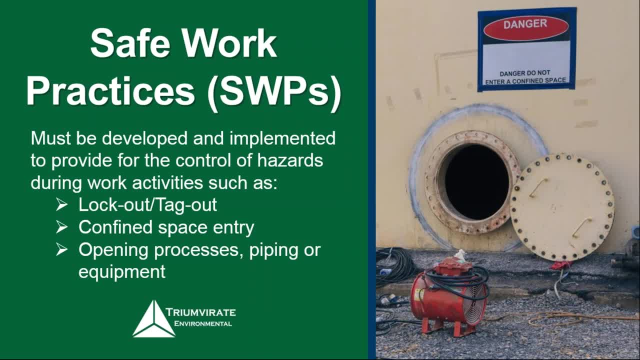 Also your emergency action plan. So I could go on and on and on here about all of the different regulations that could also be part of this program that you need to think about. So when you're picking that committee That we spoke about earlier is it's very, very important that you think about: okay, these people are going to be involved at some point too. 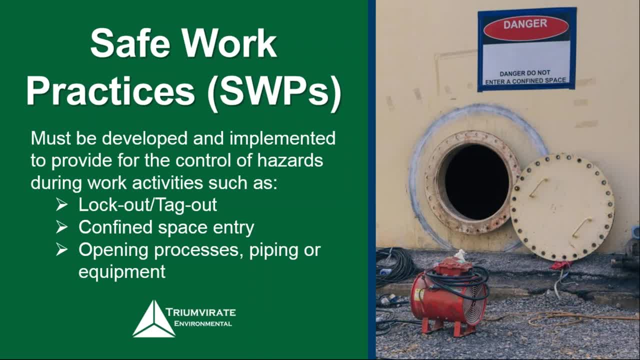 So maybe we want to get them involved right at the beginning and not necessarily at the very end- which I see in a lot of places- is because then those people feel one left out And then they tend to come in more kicking and screaming, as I like to call it right. 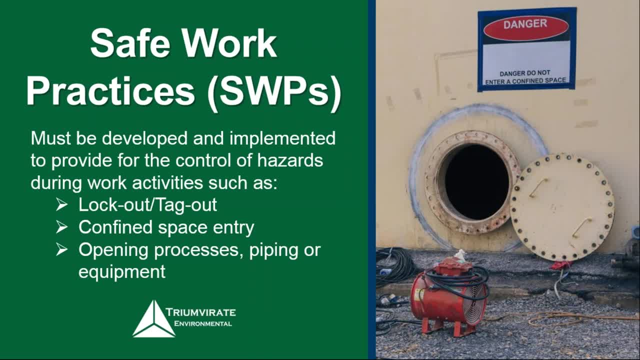 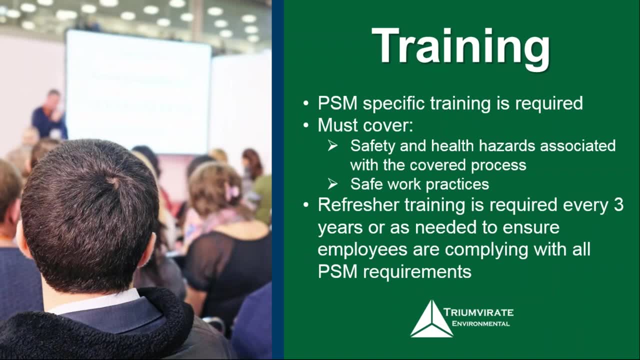 And then you lose a lot of that valuable input that they could have had to begin with. So this is a very, very important part of the process too. Then, of course, we have to do training right- Everybody's favorite thing. 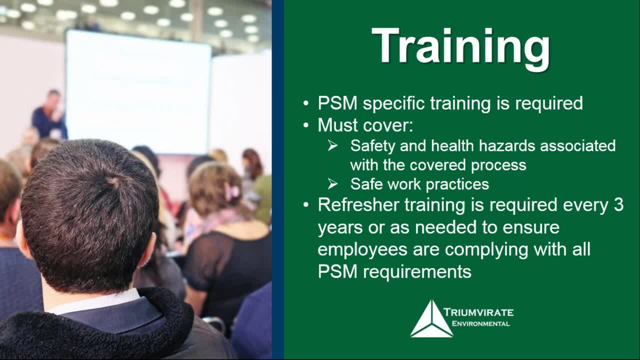 We want, you know, we got to make sure that you know, and the PSM standard, you know, says it's required. And what is what do you got to cover? You know again, you got to cover everything, that's all of the processes that occur at your facility that are part of this regulation. 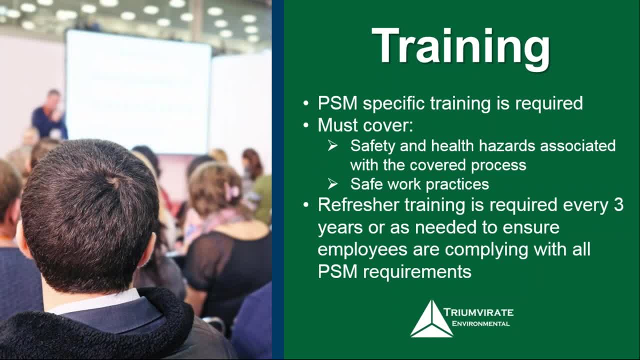 So again, we're only. you know, when you're looking at PSM And you're looking at the training of the PSM, you're really training them only to the processes that have the regulated materials. This doesn't mean you got to do, you know. oh, so everybody in the company you know we got to cover on all the hazards at our facility and all that. 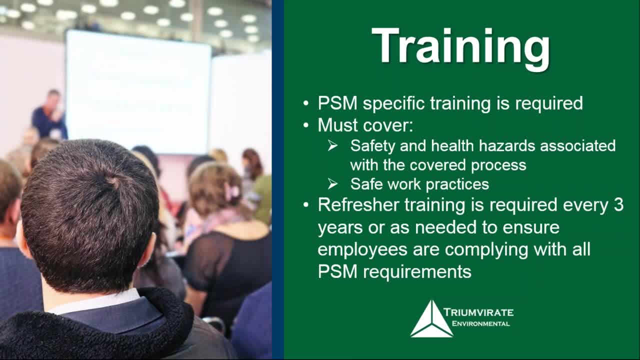 Well, I say you do, but you're doing that under different regulations, right? So you might be doing that under HAZCOM or you know, emergency action planning or something like that. This is specific to say: okay, we need to make you aware. 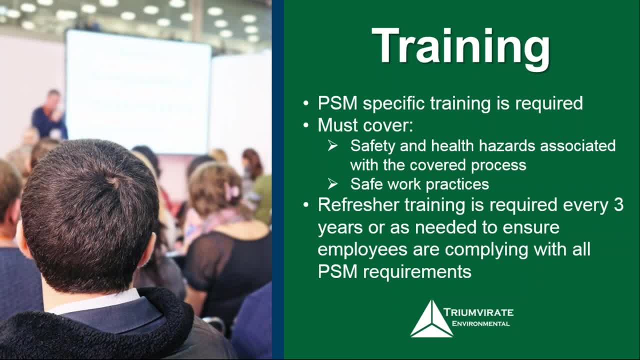 We have a PSM standard. We have a PSM regulated process here at this facility. We have it for this chemical. This is why it's for that material which is around. again back to the toxicity And we did a process hazard analysis. 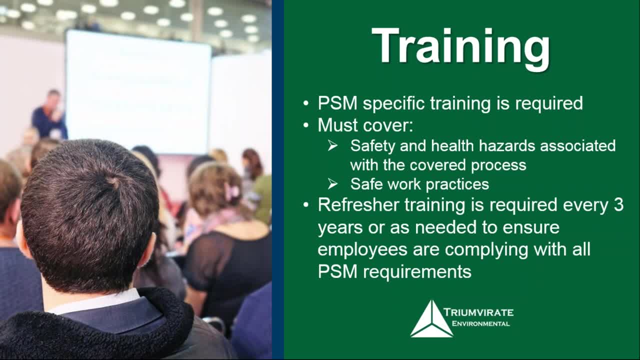 And if, God forbid, something went wrong, this could happen And we need to make you aware of it, so that this is all rolling together and everybody knows about it. And, as you can see here, it says: you know you have to do this refresher training at least once every three years. 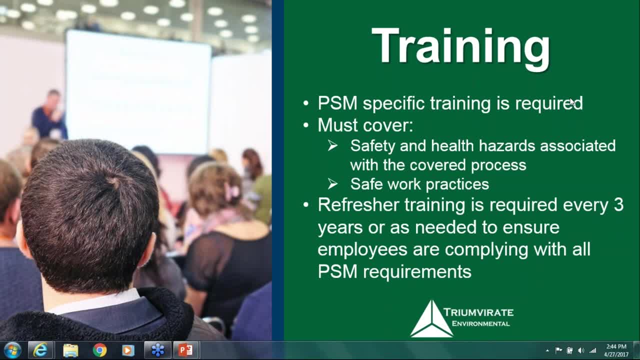 Or if you find during your annual audit- right, because I'm going to call it an annual audit, but you saw earlier how to do the review of all of your procedures and things like that- that it's not being complied with and that you're finding issues over and over and over again, then really you've got to do more frequent training. 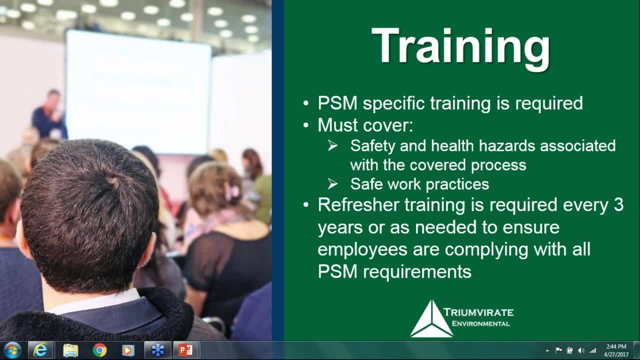 You know I've had clients that will say, oh, we do it on an annual basis. Great, if that's what works for you. But it really comes down to, you've got to look at yourself and your own facility And say: okay, you know, this is what I'm doing and why I'm doing it. 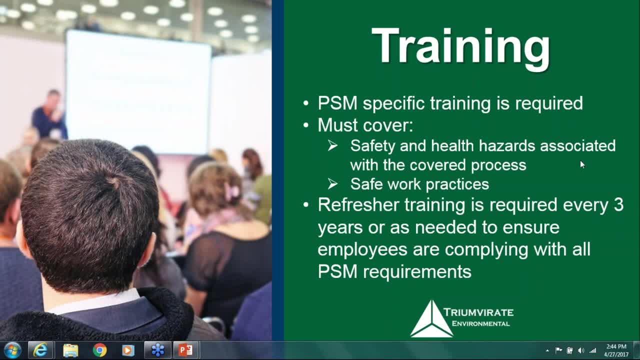 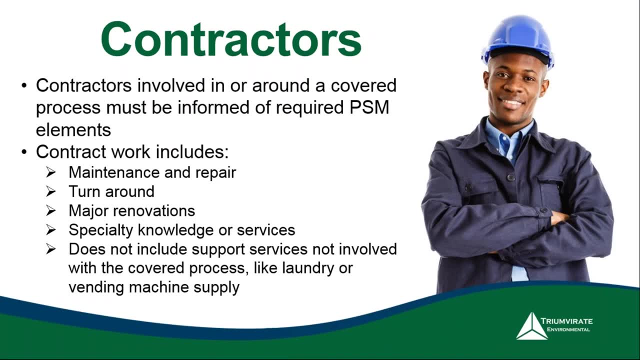 And everybody's favorite right is: we've got to, you know. the next- sorry, a little difficult bit is contractors, right. So we've got to make sure that they know what's going on because we may bring in contractors here to you know. 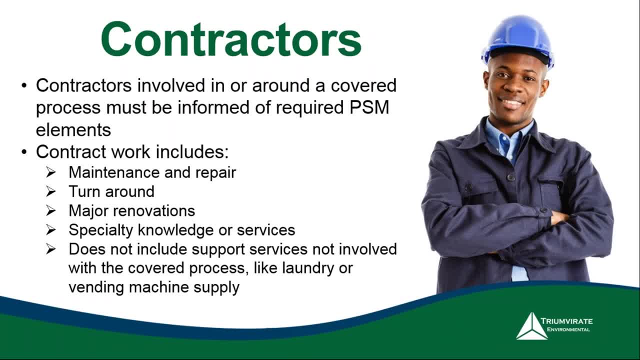 to work on these types of processes but we need to inform them. Very similar to like confined space entry right. We've got to tell them all the hazards that we know. We've got to talk to them about what do we know about it? 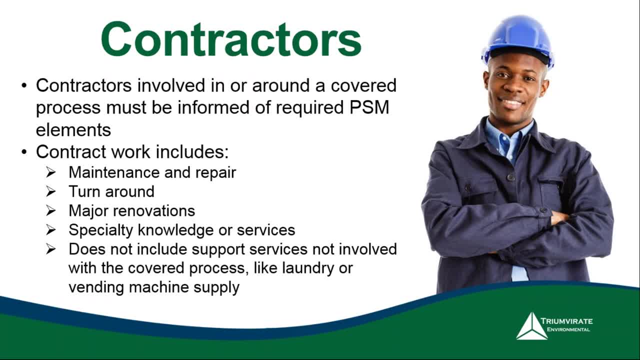 Hey, we've got to give them the training right. Sometimes it's more of an abbreviated training. I've seen abbreviated training just for contractors And I've seen them go if they're required to go through the regular PSM type of training that every employee goes through. 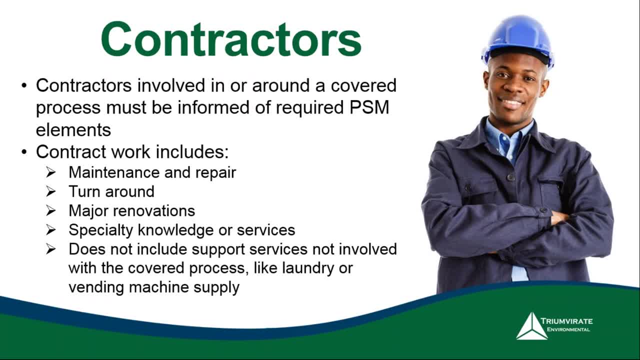 that's affected by that process. So it really, again, they allow you to do what it is, what you want to do with it, to understand and make sure that it's covered, like you know, with everything that's needed. So here is just some ideas of what we mean by contract work. 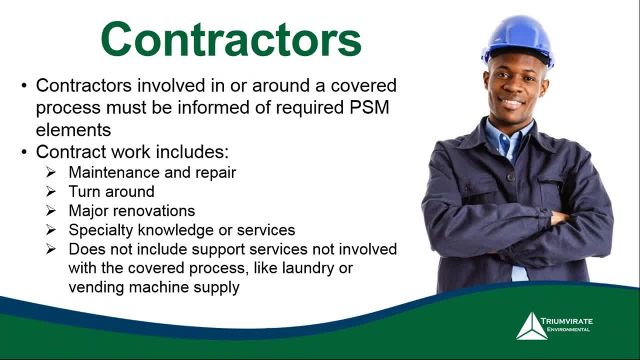 You know contractors that might do it, you know. So just you know it does not include, like it says, support services, things like that. you know that really not going to have an effect on the actual process of that system. 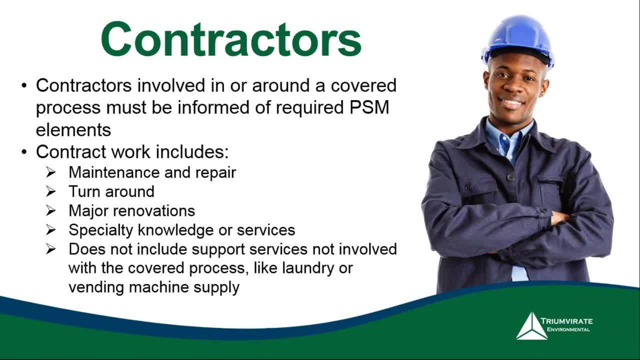 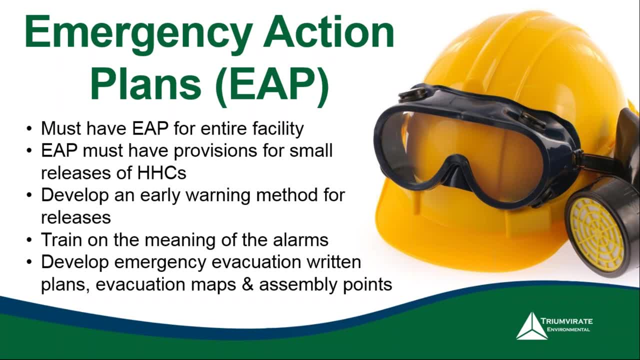 So it's more around. you know the real heavy duty type of work. Of course I mentioned this earlier. right is that you've got to have you know. obviously you've got to have an emergency action plan, right. 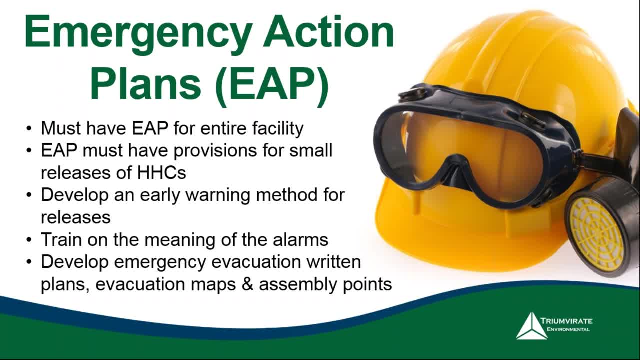 Under OSHA, every facility needs to have some sort of an emergency action plan, right, And in your emergency action plan here, this one is going to get a little more beefy, if you will. is, then, what a typical one would be if you were not in the PSM program. 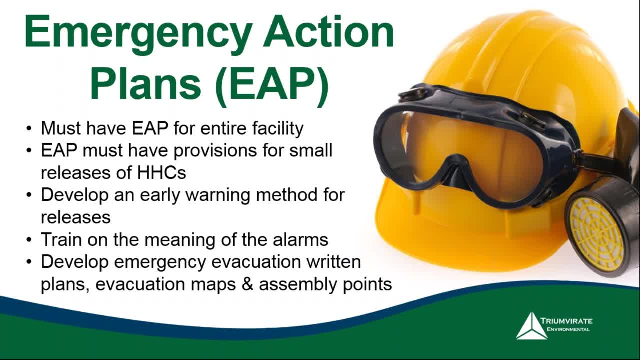 because you've got to have it for you, You've got to have it for the whole facility And it's got to have in there for you know. it's got to have the provisions in here if you had any small releases of the high hazard chemicals. that's what HHC says. 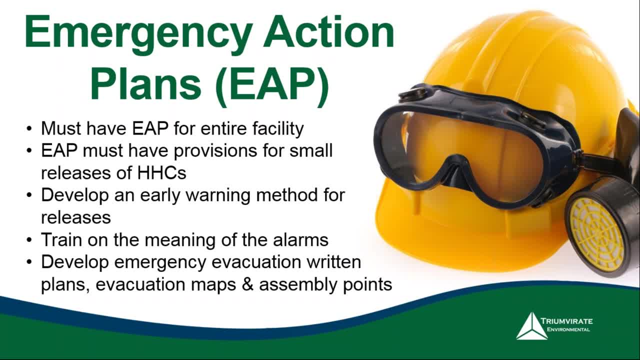 is highly hazardous chemicals that we talked about earlier And you've got to have in your EAP is it will talk about. what are you going to do? what types of early warning methods do you have in case of a release? And that could be anything from an audible alarm to you know, strobe lights to you know. 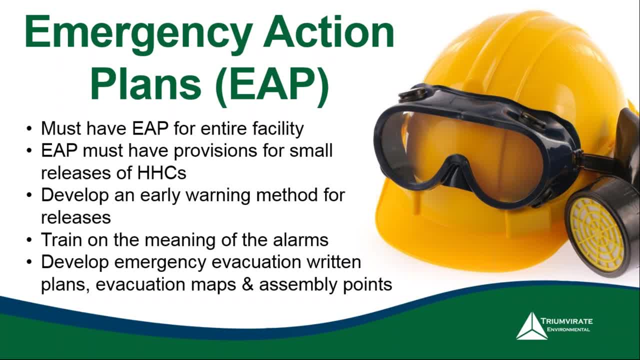 whatever you're going to use, is it PA system? is it you know like? and then we're going to talk about what? about the? you know the evacuation plans? How do you do that? Are people going to get out? 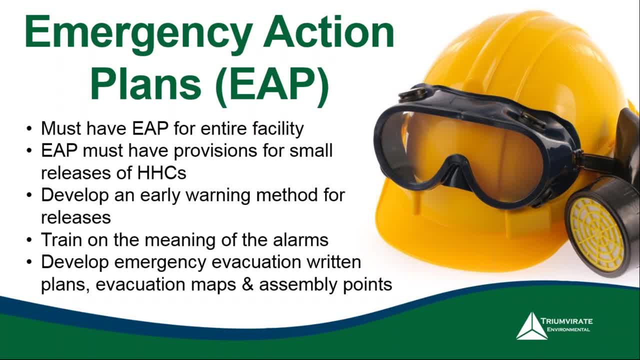 Did you think about: okay in your plan? did you think about: all right, this process could actually, if it ruptured and it leaked, it could actually go into one of those. Well, that's got to be documented. You've got to have a plan to say, oops, okay, we're going to have to redirect people to a different route. 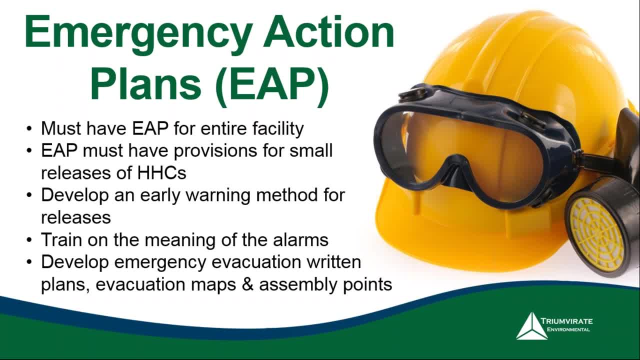 to ensure that they're not literally going right through the release area. So these are some of the things that you want to get you know, put into consideration here And, you know, make sure that, as we all know today, you know the one above that right. 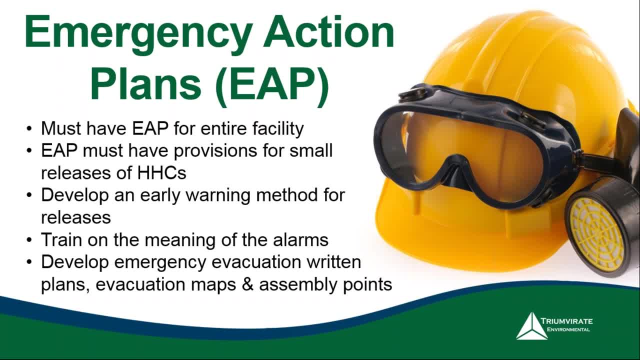 is trained on the meaning of the alarms is because, I'm sure some of you will shake your head- yes to this is when we pull the fire alarm, or my favorite word for it is the evacuation alarm right. what do most people say? 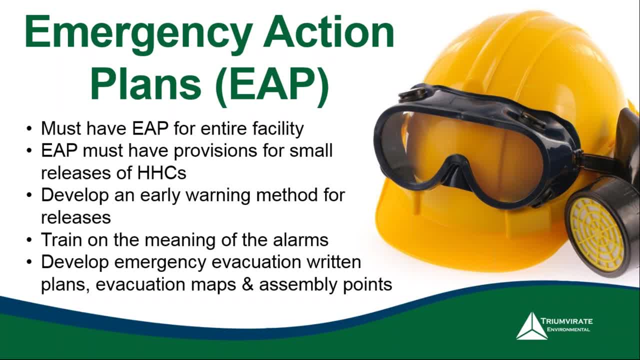 Oh, it's just a drill, No big deal, right? Or if it's raining out, really I've got to go outside in the rain or in the snow, or right, most people take it. you know, too nonchalantly that they don't take the necessarily the, you know. 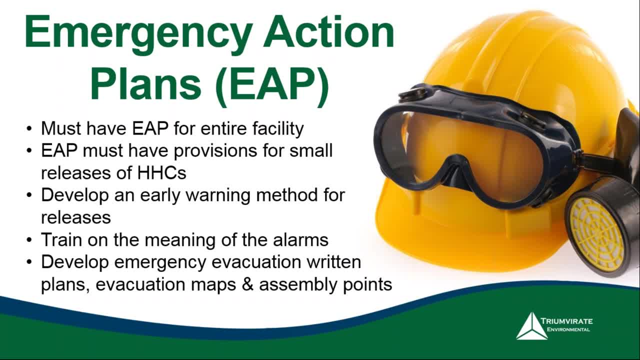 real importance of getting out quickly, that you really, really want to stress to them that if we had an alarm in one of these you know processes that are involving the high hazard system, involving the high hazard chemicals, really want to get out and get out quickly. 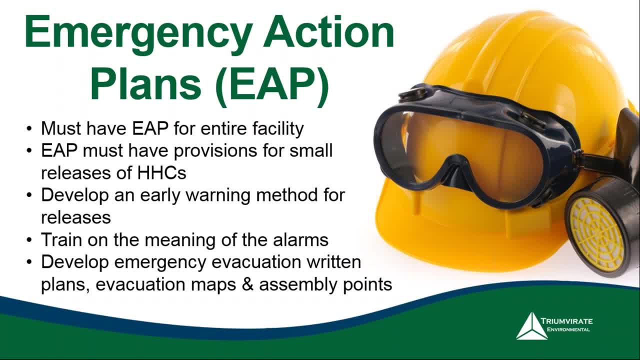 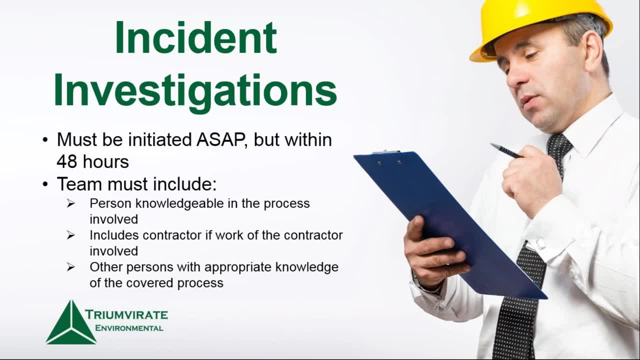 So you can't take that for granted that it may be just a drill. So it's very, very important that you instruct your employees on that front. So from there, if again, if something happened at your facility, okay, you have to, you must, you must, you must. 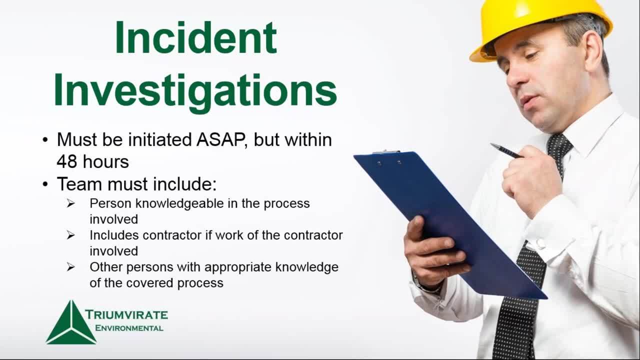 as soon as absolutely practical. you have to start, you know, the investigation into saying what went wrong. Why did it go wrong? Where did we fail? Right, Because you should have already known what could fail and you should have been looking for why it could have failed. 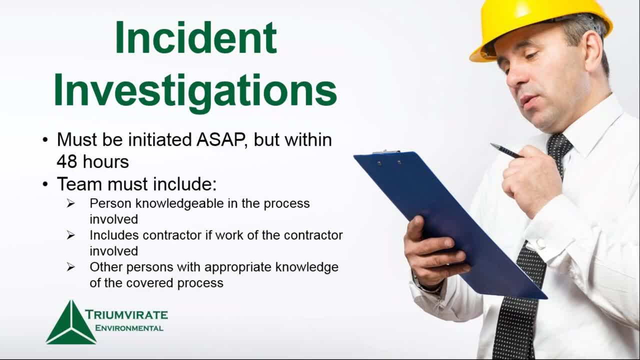 So you've got to set up again. you notice, here with this program it is a lot of teams. As I always say, I like to call it the process safety. you know management, it's PST process safety team. 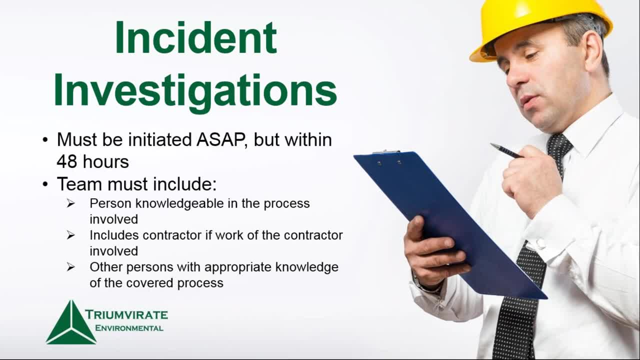 because almost everything we do is in teamwork And if a contractor was involved, then you've got to set up a team. You've got to get them involved in this. accident investigation too is- I'm sorry- incident investigation is to make sure you know that you've got all the right people in the room and that you are really sitting there. 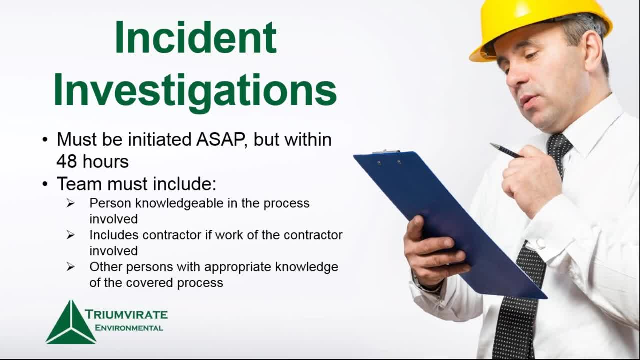 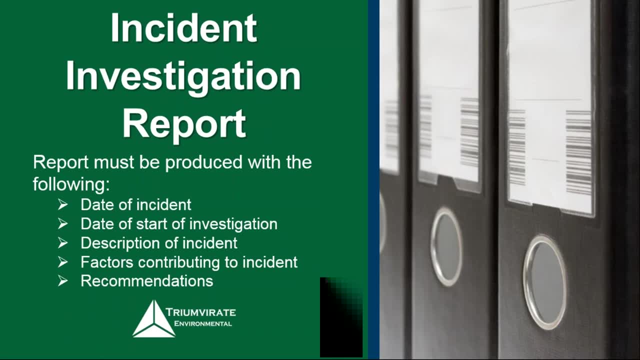 and going through and saying, yeah, we did everything we could do, And then you've got to come up with a report. So, as we said earlier, you've got to talk about what did you do. when was the incident? when did you start the investigation? 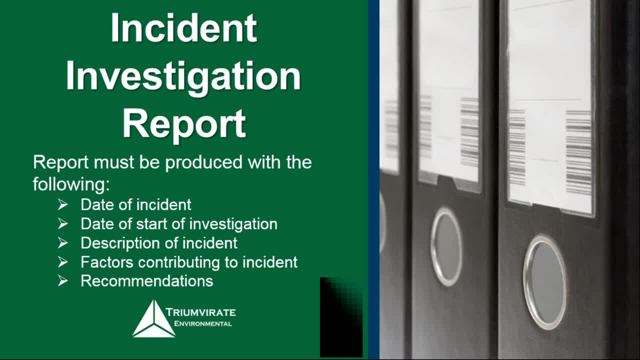 what did you figure out and, most importantly, what are your recommendations to ensure that this, hopefully, will never, ever, ever happen again? Okay, because typically when you get one of these types of incidences, it's pretty severe, It's a, you know, it's not a good thing. 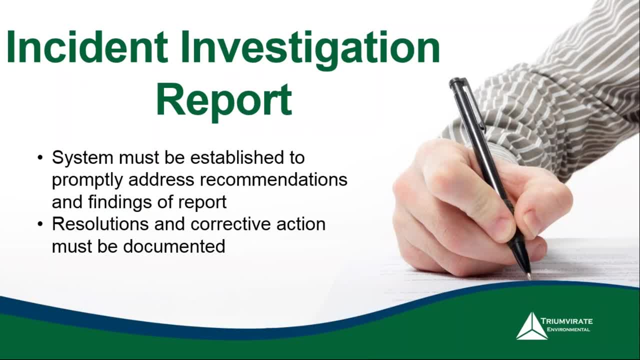 It's a very, very hard thing to look at. So also in there you have to. you know your whole system. you know you've got to have a system established as part of this. This is kind of like again- and I hate to go back to ISO, but I tend to think there's a lot of linkage to it. 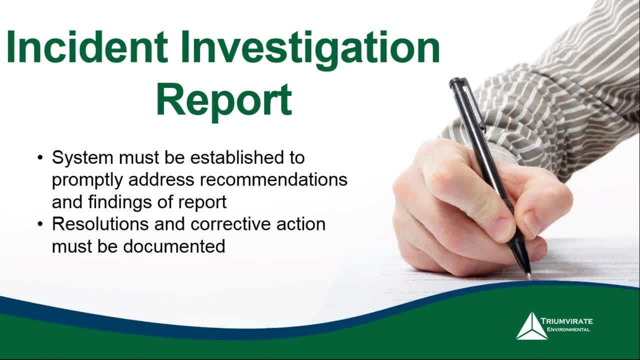 is like. you know your corrective action program. it's the same thing here. You want to make sure that. all right. how are we going to do it? Who's going to do it? When are we going to do it? 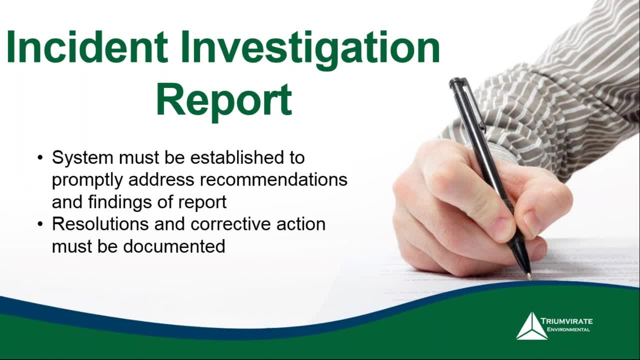 Do we present it back to our initial committee? And then how do we make sure that all of this information is processed and to make sure that everything is done right? And then how did you resolve it? And then you know how do we track all of this. 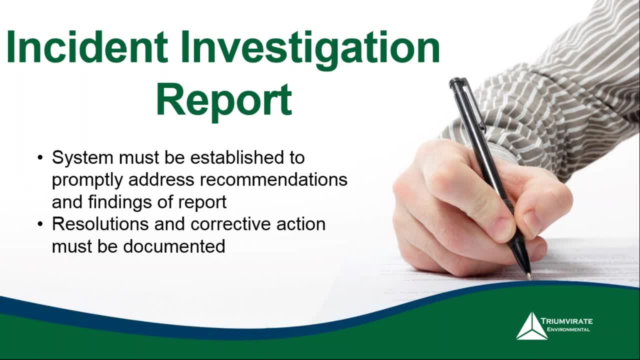 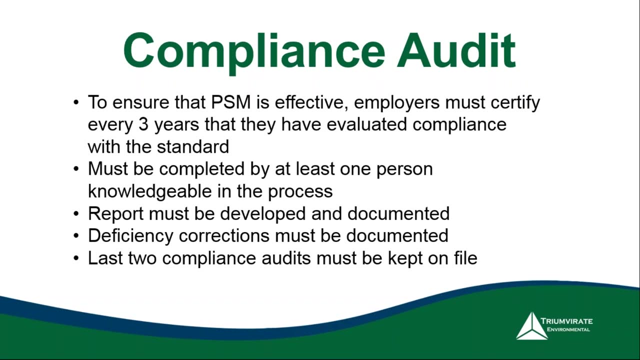 So back to the document: control right, So that plan, do check, act again, kind of, if you know that cycle, that cycle is kicking in all the way through, just making sure that everything is there. The best part of all of this right is now you get to do it in a nice compliance audit. 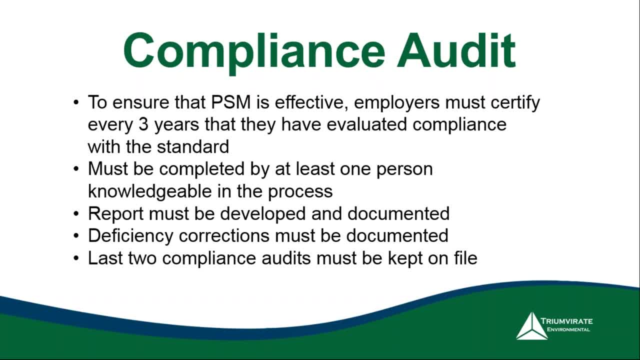 So, in order to make sure that your program is effective, right is, you've got to have it evaluated. you know, at least once every three years is to make sure to that every part of this program is complied with. You know, hopefully, right? I always stress this. 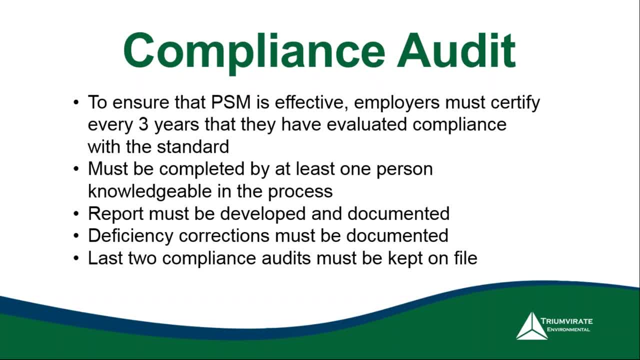 hopefully. you know you did not have any incidences and this is just really a routine. you know, check the box if you will type of an audit, which I know they're not. they're much more complex than that. 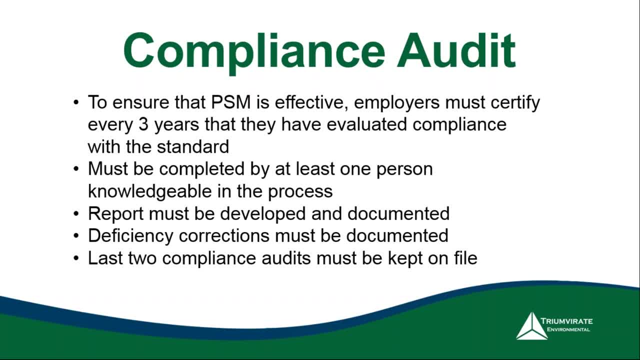 But it is really there to say, okay, what can we do, how do we do it and how do we make sure that everything is there? And in order to do this, you've got to have at least one person that's participating within the program, that's knowledgeable in the whole process. 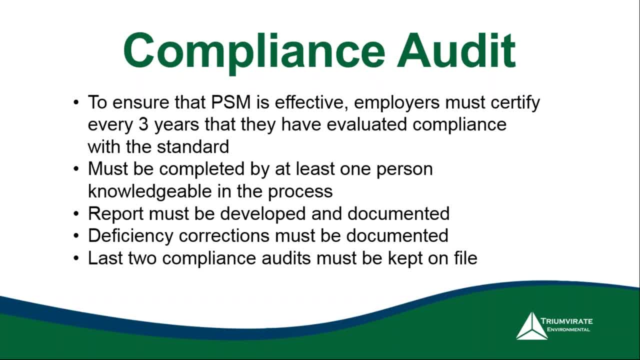 Okay, So you want somebody there that really understands how, you know what processes are affected, how are they affected and why are they affected. You want a part of the audit program. Okay, You've got to have a report and you've got to show that any deficiencies that were found must be corrected and then documented. 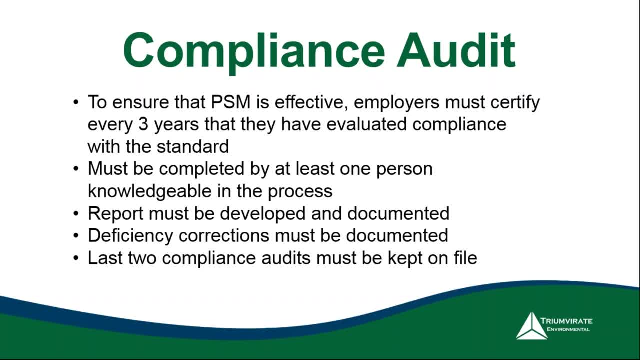 And you've got to have the last two compliance audits must be kept on file. So that really means you've got to have what like six years, right? So you've got six years, you know two cycles, which is six, right. 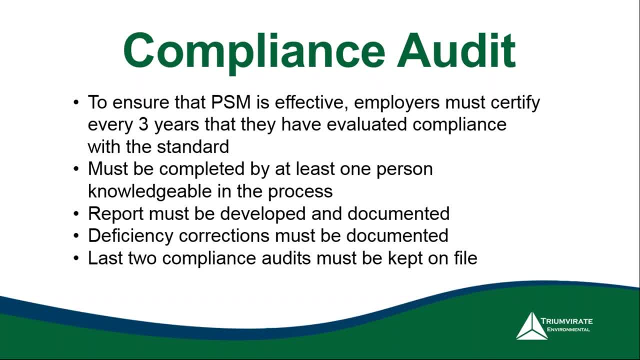 So you want to make sure that you have those in place for yourself. or, if you know, OSHA came in and they did an audit of you- that you have these documents in front of you. Very, very, very important thing- And I always say you know to everybody too- if you do an audit, is you know what? take a look at it. 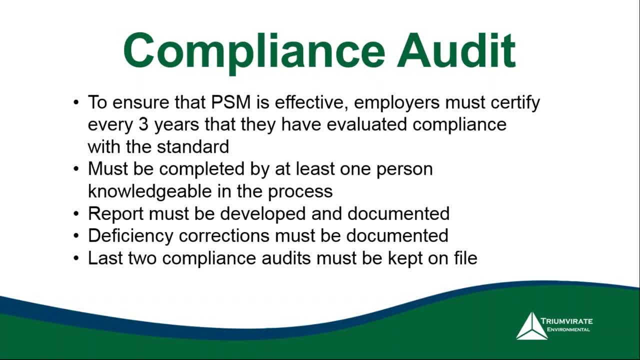 Maybe you do the full-blown three-year- you know heavy-duty compliance audit. but it might be helpful too, maybe on an annual basis, to go back and say, hey, we had an issue here, Let's take a look at it again. 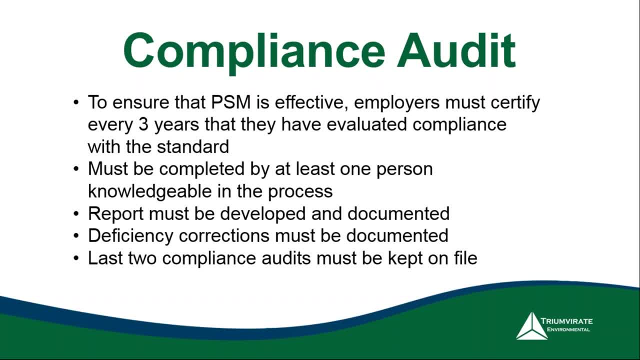 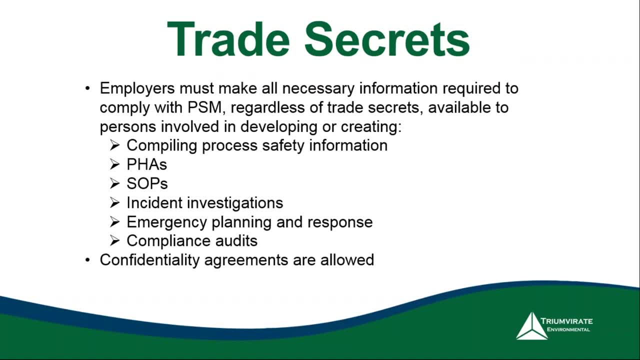 Let's make sure it hasn't creeped in again. Why wait until the three years to do the official audit, if you will? There is a piece in here too, kind of getting close to the end here. I know I'm getting very close on time. 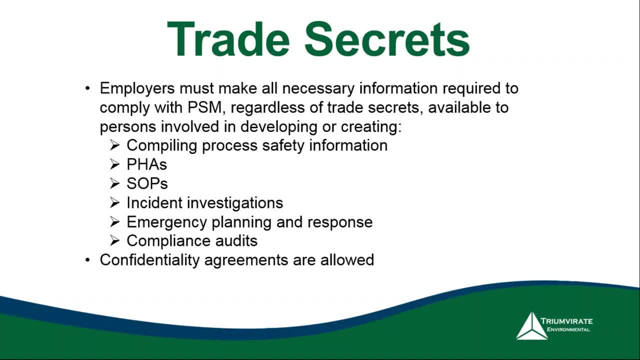 So here's trade secrets too, And also make sure that you know it does allow in here. you know that you can take you know into consideration, that you know some things are trade secret. but they say: you know what? 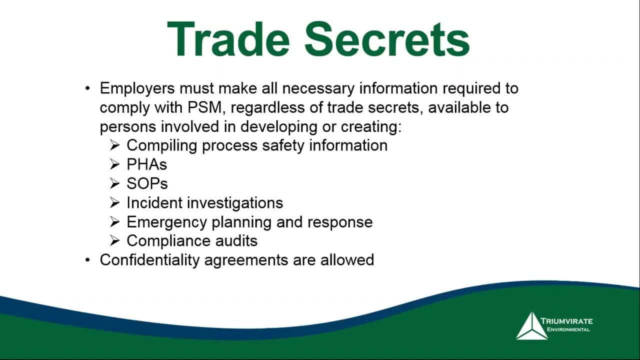 You've got to make sure that You can't claim that, And you know I was talking to somebody recently. oh, we don't have to do that, We're covered by trade secrets, Like no, you've still got to follow all of the regulations and all of the parts of the rule. 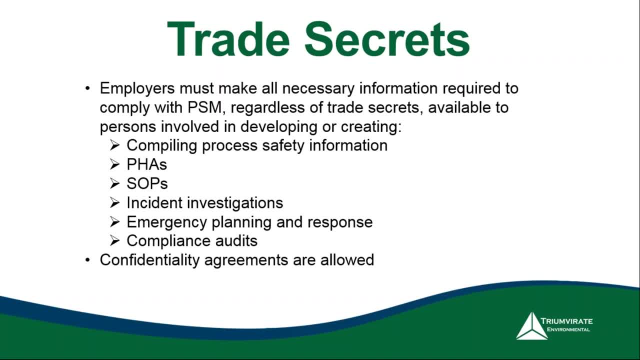 It's just, you know, you can put some confidentiality to some of it, but you can't just disregard it because you are, you know, claiming a trade secret for this type of a process. So it is very, very, very important that you look at all of this. 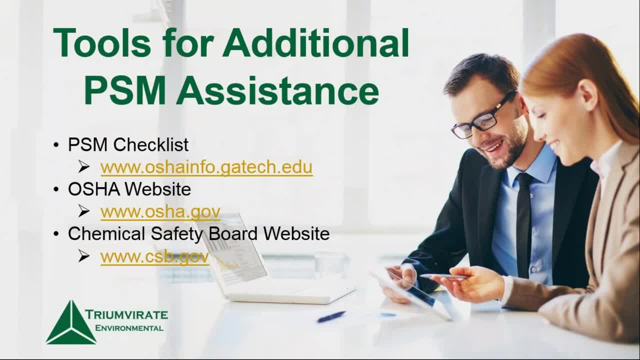 So, with that in mind, as we said, we just really went through a whole pile of stuff here, And there's a lot of good information out there. You know there is a process safety management checklist that's put out by Georgia Tech. 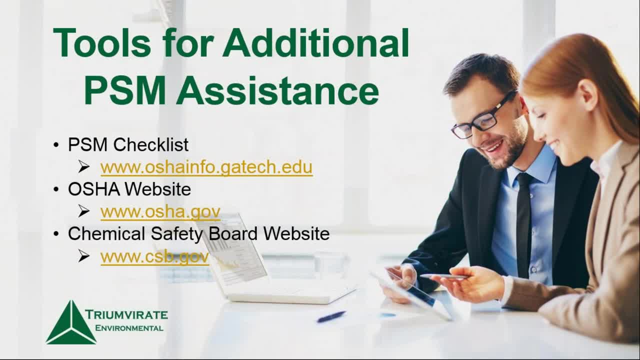 You know we have a link on here for you, Obviously, the OSHA website. The OSHA website has a ton of letters of interpretation, as letters of interpretation really are there to tell us how does this stuff work, what do they really mean, what is the purpose of it. 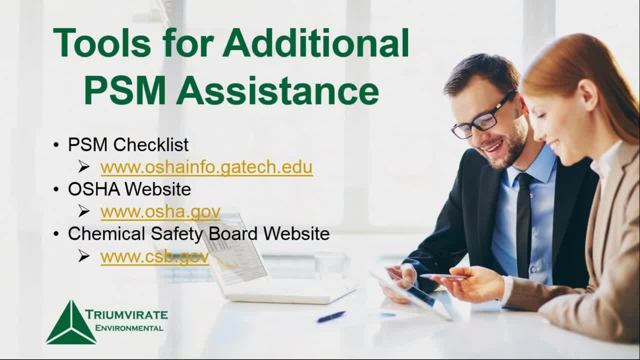 And things like that, And one of my favorite websites- even though I always say we go there for the wrong reasons, right- is the Chemical Safety Board, you know website, because it actually tells us about real incidences And it's great because if you have a similar process to what somebody is doing, you can actually, you know, learn from their mistake if you will. 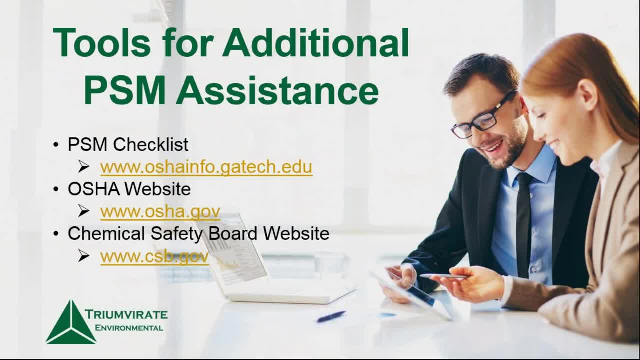 What I mean by that is you can go in there and it will actually show like to say: oh my God, you know they have this catastrophe, But this is what we think the reason why it happened. And hopefully you can take that information and go back to your own facility and say: okay, you know, let's look at that in a bigger, in a different way and say, hey, could that potentially happen here? 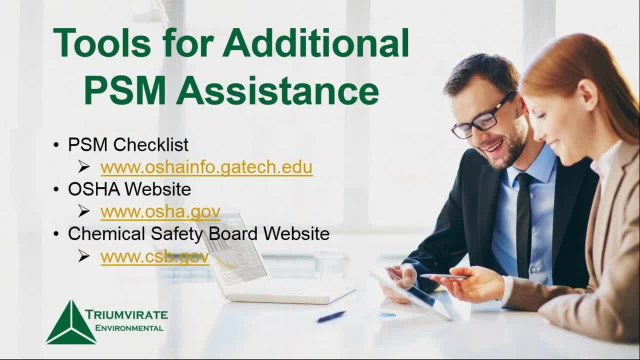 Could this happen this way or that way? So it is something that we want to you know, share with you and say that is a great resource in which to look at. So with that, James, I am going to switch. Thank you. 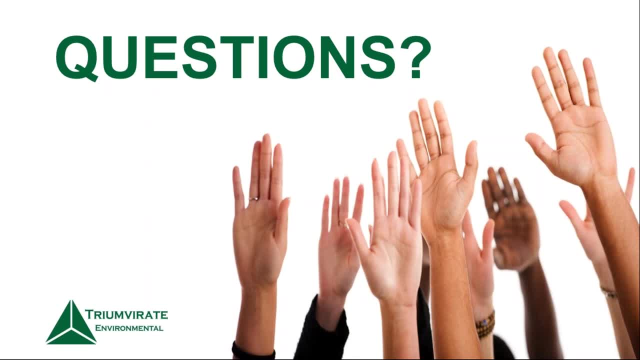 And I'm going to switch this over to you for questions. Great Thanks, Rick, And we do have a few minutes left for questions. I didn't see very many come in, But I want to remind you to type in your questions. 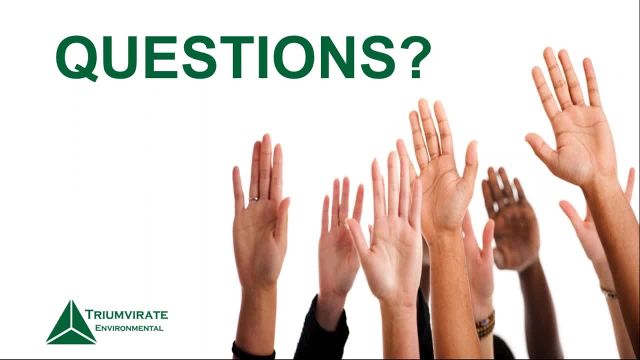 And if we don't get to it right now, I'll make sure Rick and I touch base afterwards and we'll get you some responses for that. So while Rick catches his breath, I think I'm going to just run through a few conclusion points. 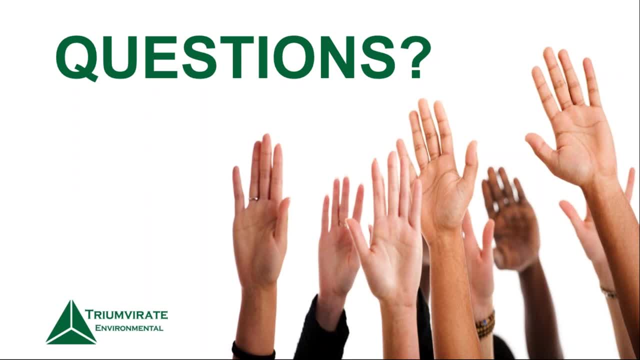 If you missed us at the top, I want to let you know that you will receive a copy of the slides and a recording of the webinar, And that will arrive in your inbox tomorrow morning, So keep an eye out for that. We'll also send a link to a short survey. 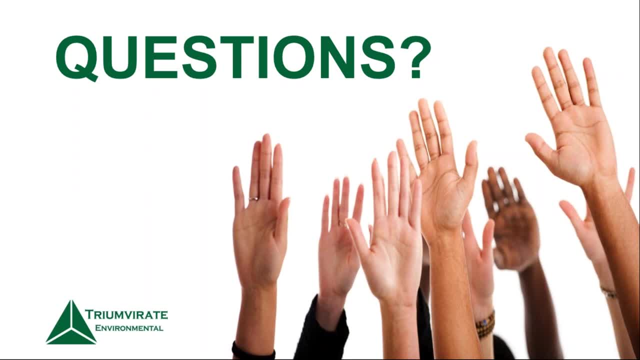 We'd appreciate your feedback on the webinar, ideas for improvement and ideas for future topics, So let us know what you think. Also, as a thank you for attending, I mentioned we would make an offer at the end for a compliance review. 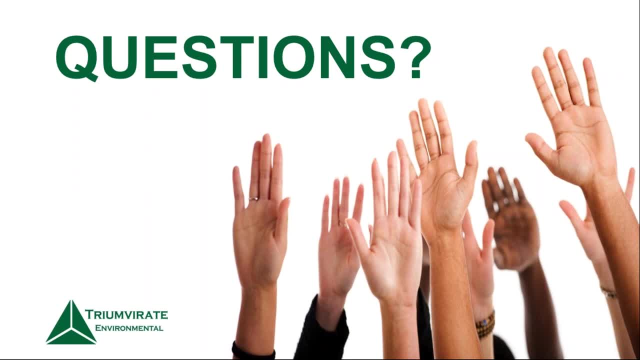 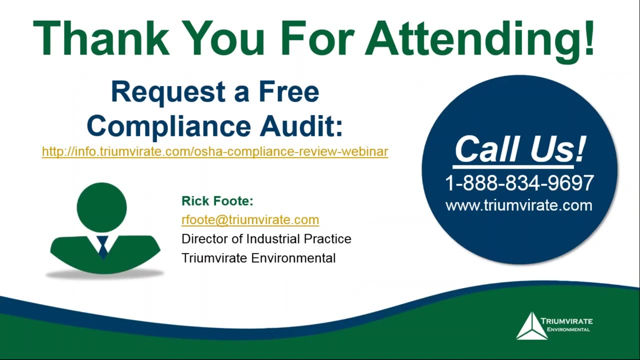 I'm going to shoot that over in the chat box. if you're interested in learning more about this complimentary OSHA compliance review, So take a look at that While we're still on the line. And also, Rick, if we can advance to the last slide, I want to share your contact information with the group. 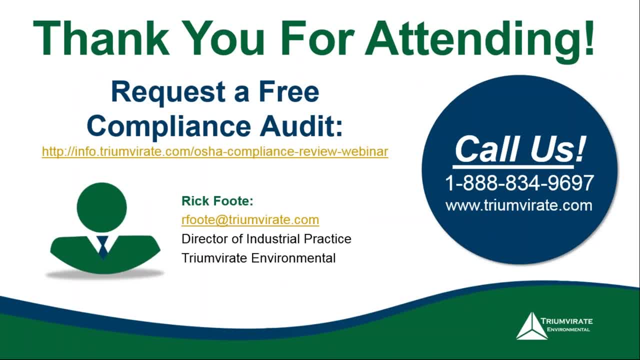 You'll see Rick's email address. I'm sure he'd love to hear from you. And if you want to get in touch with Triumvirate, our phone number is listed there. So a few ways to get in touch with us. 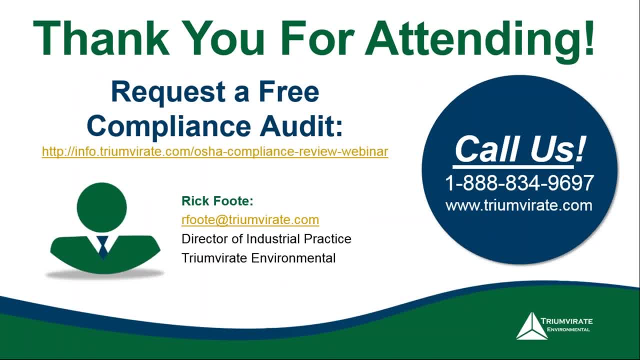 If you have any questions, let's get those in. Otherwise we can probably close down in a couple of minutes, But I'll take a look and see if anything has come in. Yeah, lots of questions about getting the slides. So I know Rick presented quite a bit of information today. 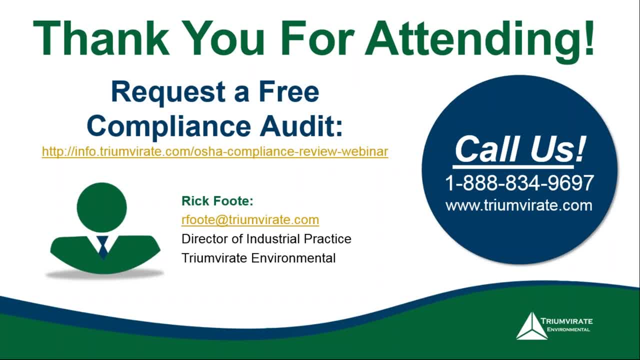 So I'm sure hopefully you weren't jotting down too many notes, because you will get this. But, Rick, I think we can conclude. We've got two minutes here. Do you have anything else for our audience today? No, I just think you know. obviously, as most of you may know, OSHA has been very, very active. 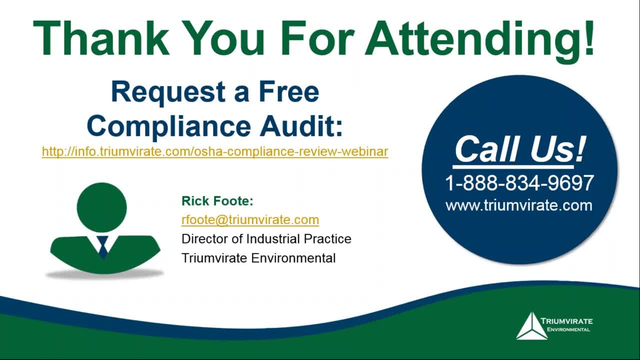 You know, This is just one of the topics. The new, you know, slip strips and falls right has just kicked in. So you know, really just pay attention. And really the key to this program here is that chemical inventory and, you know, determining if you have anything at your facility that may be, you know, trigger these requirements. 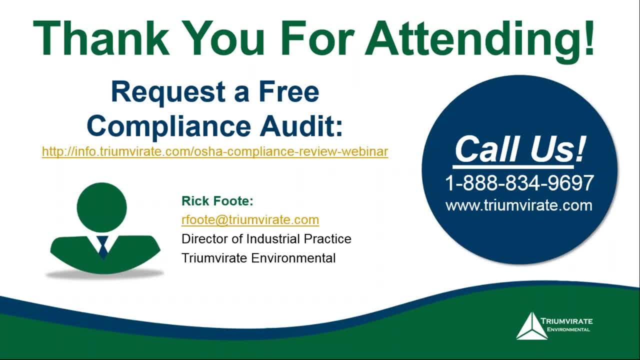 And you know you really just got to follow it and make sure that you comply. So make sure to keep your employees safe. That's really what it's all about. Awesome Thanks, Great advice. Next question: As a plant comes offline, Rick, when does PSM no longer apply?